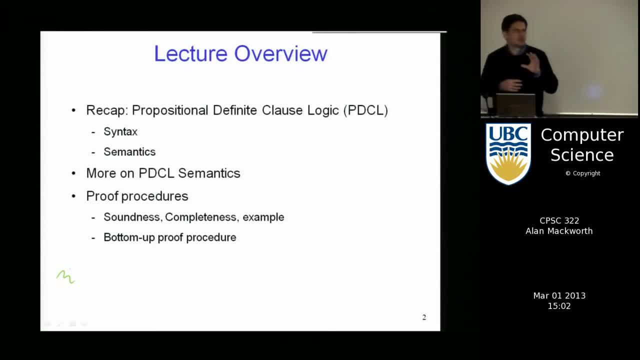 So all these steps are steps that you need to perform for any logic. So if you understand them on this basic, simple logic, it's going to be much easier to generalize to other. Okay, So let's go back to revise a little bit what we saw last time. So we are looking. 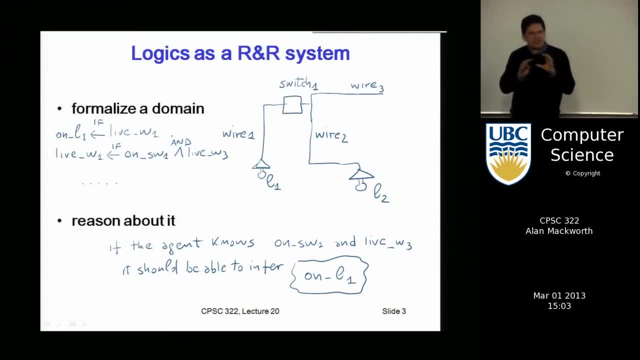 at logic as a representation and reasoning system. So we are not trying to model like mathematics. We are not going to build a system of logic. We are going to build a system of logic. So we are going to build a system of logic. We are going to build a system of. 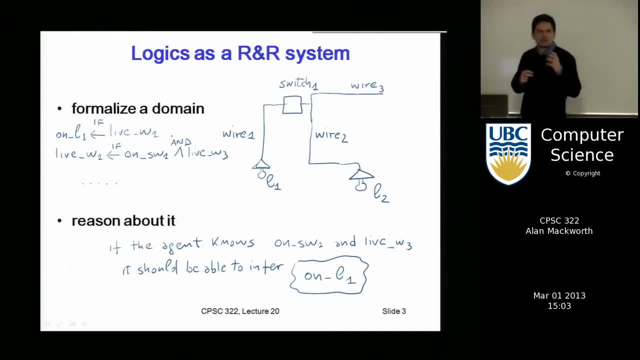 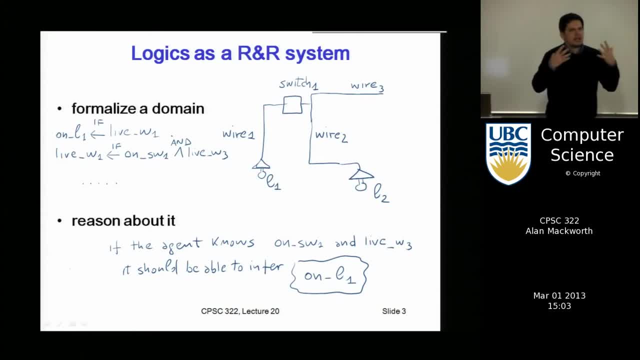 at the possible, like possible war, And we have to decide what of the objects we care. So in this example you have like wires and switches and lights, And then you have properties of these objects and true or false. So these are the propositions, And then we state: 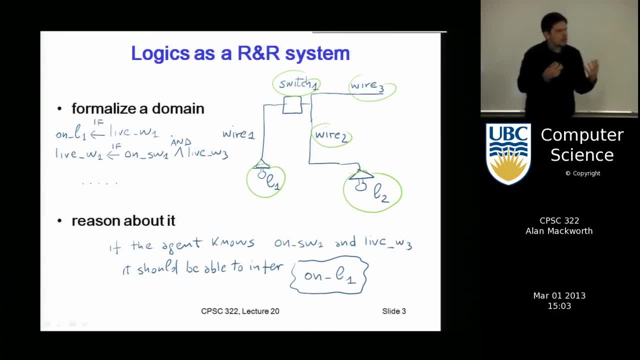 We make statements about connection, logical connection between these propositions. For instance, we can say that the light is, light one is on only if wire one is live, so if there is current here. Or we can say that the wire one is live, there is electricity only if the switch is on and 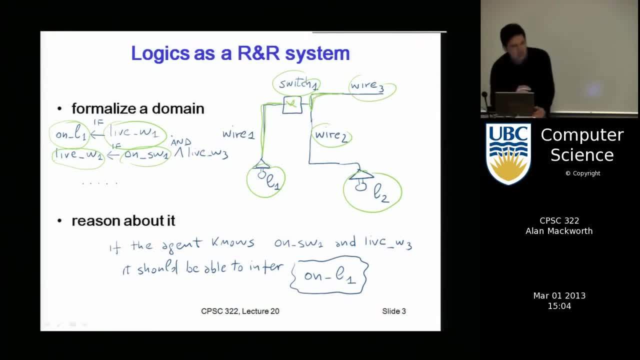 there is electricity on wire three. So you can describe the simplest circuit, you can describe your world with propositions that can be true or false, and then connections between these propositions, between the truth value of these propositions, by using logical forces. That's what you do when you represent. so formalize the domain or you represent. 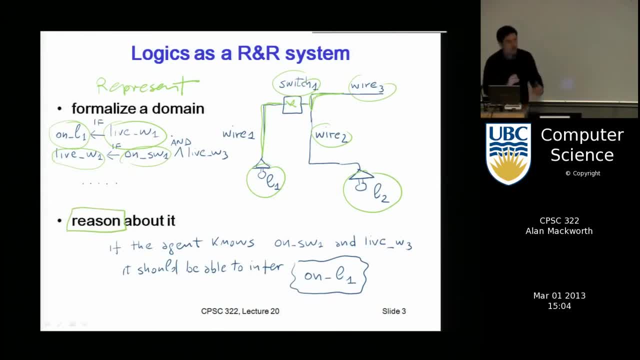 But then you want to reason about it. so the goal of logic is to reason about it and you say what can be true or false. But then, given that you know that something is true, so a subset of the propositions are true. so in this case the switch is on and there is current. 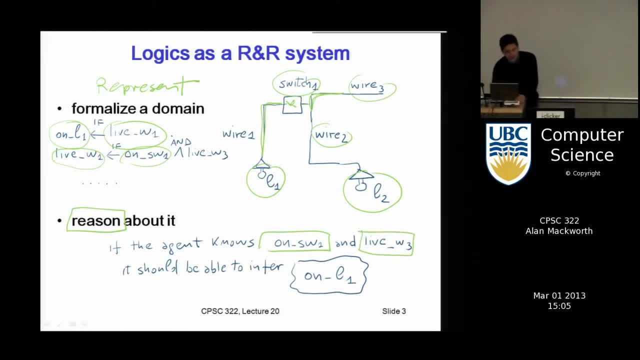 on wire three. you want to be able to derive. what else should be true, given what I already know? So the goal of logic is to develop a way to do this effectively. So we are going to see that. So we are going to see today a way to do it that is semantically sound. You can see. 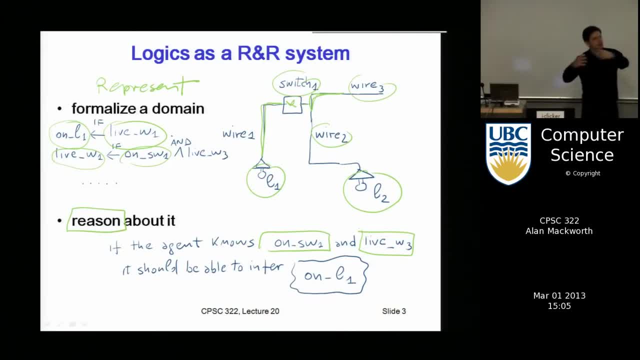 why you should. if you believe something, you should also believe that something else is true. But we are going to see that it is unfeasible, that you need to devise what are called proof procedures that can do that in an effective way. 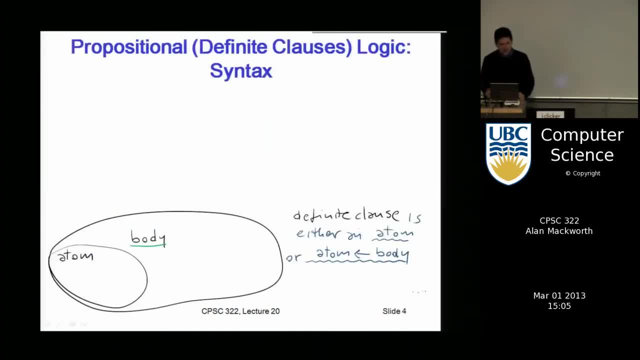 And, as I said, we are going to work with a very restricted form, in a restricted form of propositional logic. So in propositional logic you have only this proposition. that can be true or false, but you can use all the logical operators that are available, like 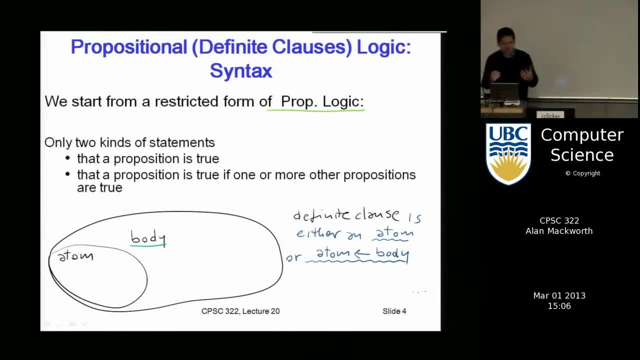 the negation, the OR the AND. So in propositional logic you can write expressions like P1 or P2, negated if and only if not if-free, And P4. So you can create these formulas. Those are the ways in which you can specify constraints. 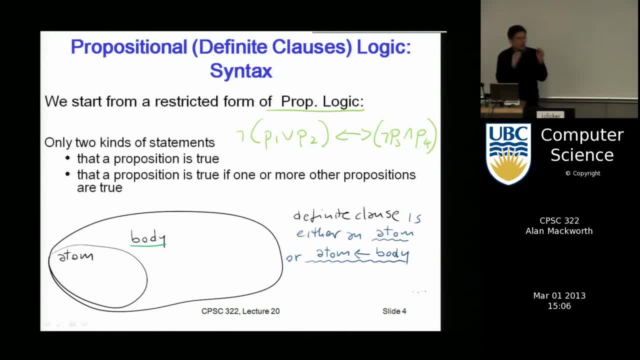 on the truth value of this proposition. We are looking at the subset of this language so that we can understand how you define the semantic of a logic, how you define logical entailment, how you define proof procedure, how you prove stuff about the proof procedure. 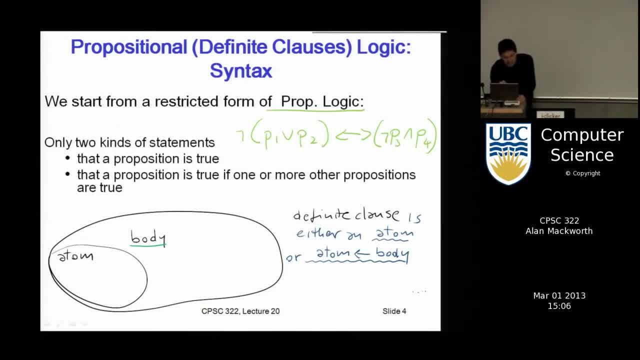 So what is this simplified version? This simplified version is definite clause logic and we saw last time you can just say that a proposition is true or false. So you have atoms like P1, P2.. So the building blocks are the same as propositional logic. 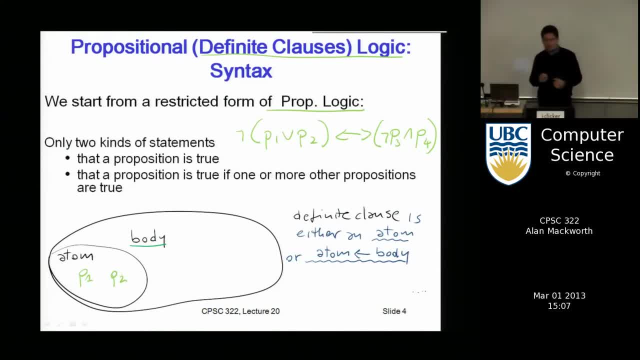 Just symbols that refer to something that can be true or false. Then you have a body that is just a conjunction of atoms or an atom just by itself. So the body can be P1 and P2. And P3. And then a definite clause is either an atom, it's either just a proposition. 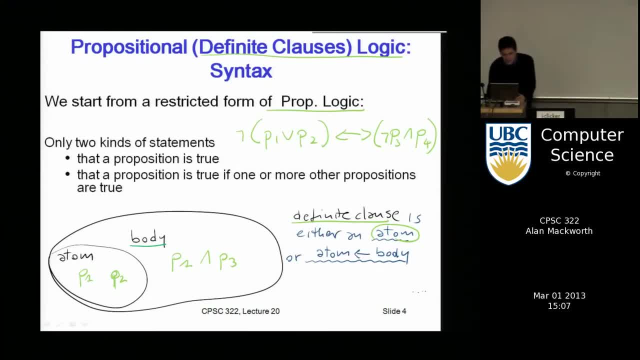 or a rule of the form atom implied by a body, So it could be something like P1, or P3, and P4.. Okay, So in this language, your knowledge base is only being a subset, a set of definite clauses. 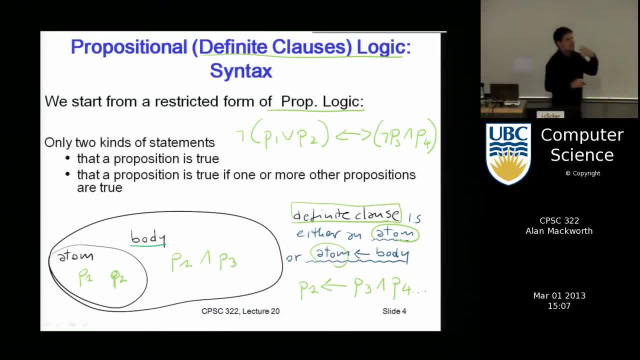 So your knowledge base is just a set of either atoms, like propositions that you say are true, or rules in which you have the antecedents in the body and the consequence they had is just an atom. Okay, So this is what. 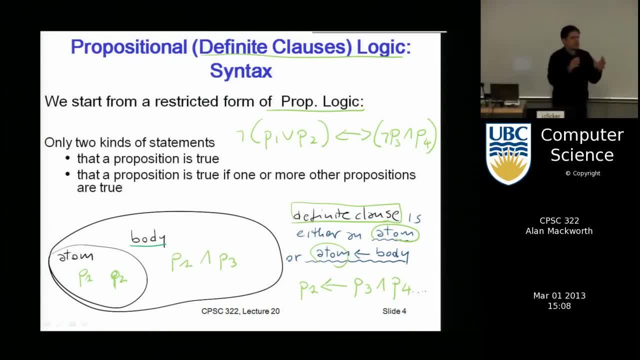 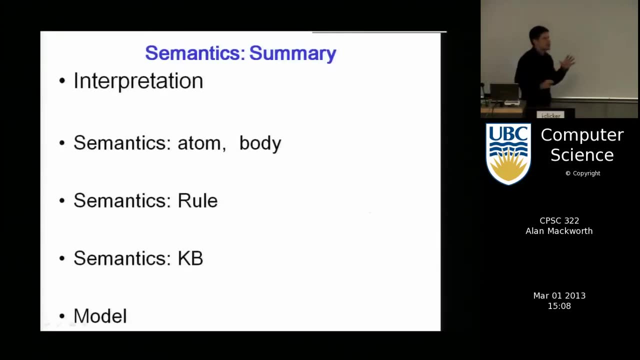 It's the syntax of our language. It's just what kind of statements we can make. We can just say a proposition is true or a rule is true in the knowledge base. Okay, So now that provides the semantics that we most of it. we saw it last time. 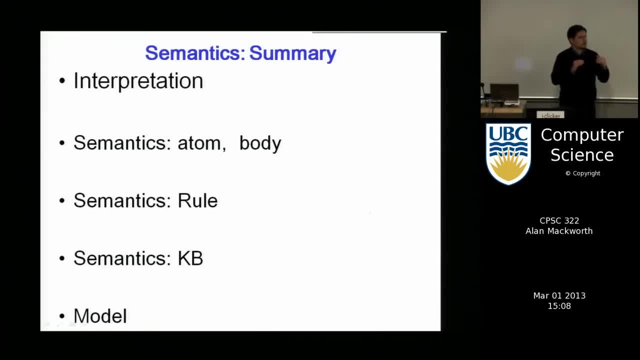 So, in order to establish whether a formula like either an atom or a rule is true or false, you need to refer to a particular state of the world, Okay, Which is called an interpretation. So let's assume that you have four P, Q, R, S, four propositions in your environment. 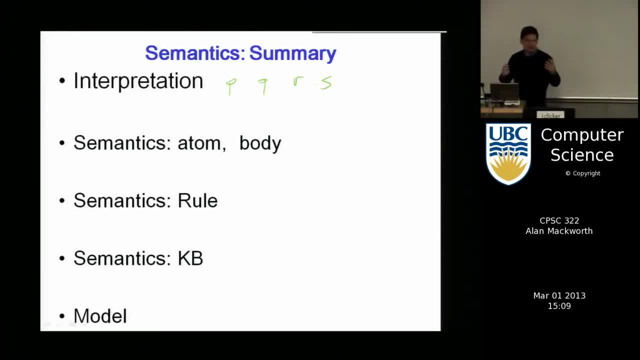 which obviously is not realistic In a realistic environment. there are thousands of these, But if you have four propositions, how you can describe a state of your, of the world, a state of the environment? Well, you need to tell for each of them whether it's true or false. 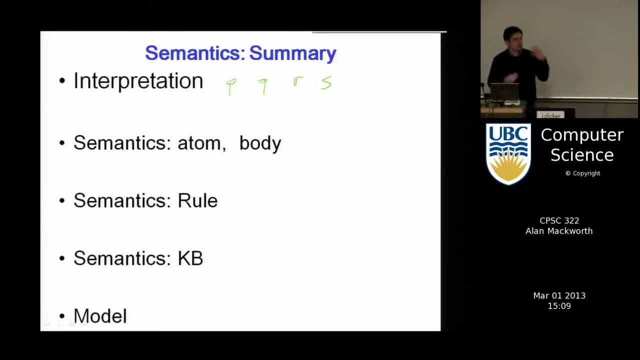 So any possible assignment to the, to your proposition, to the symbols, to the atoms, is an interpretation. So one interpretation could be that P and Q are true and R and S are false, or true, true, true, false. 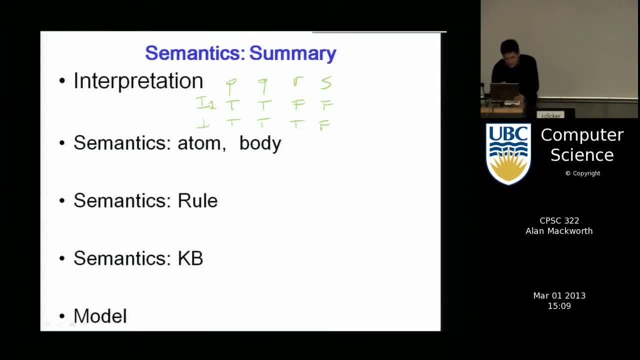 So each of them is an interpretation: E1,, E2.. And obviously if you have N propositions, you have 2 to the N interpretation. Yeah, We're not allowing the binary values of true and false correct. We're not allowing any other values in this picture. 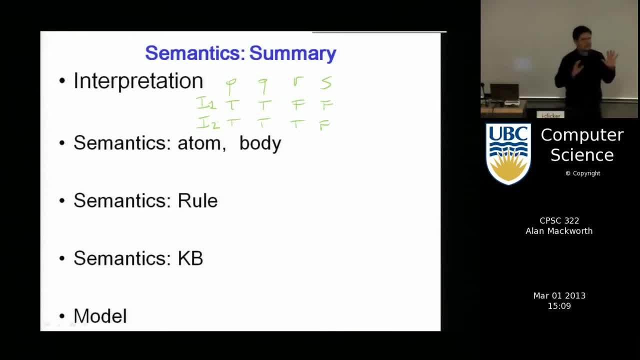 In propositional logic it's only binary. So they're binary, they're binary variables. And now that you, you decide, I'm in this environment, in this specific interpretation, well, you can now define whether an atom is true or false. 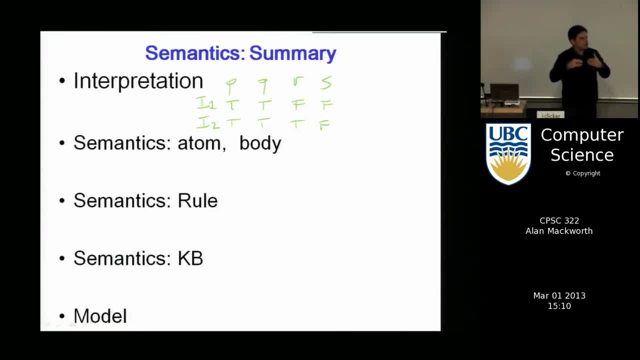 Whether a body is true or false with respect to the interpretation, Whether a rule is true or false with respect with respect to the interpretation. So for an atom? well, what about the atom P, with respect to the interpretation you want? Well, you just read it, it's true. 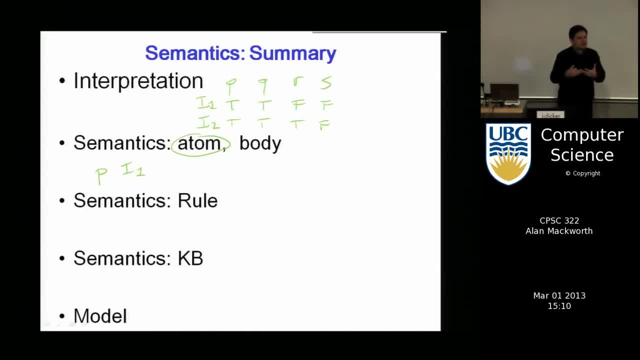 Okay, So for atom it's straightforward, Whatever the interpretation is telling you. that's what is the, the semantic of the, of the, of the atom For a body? let's say that you have N propositions, You have P and R. 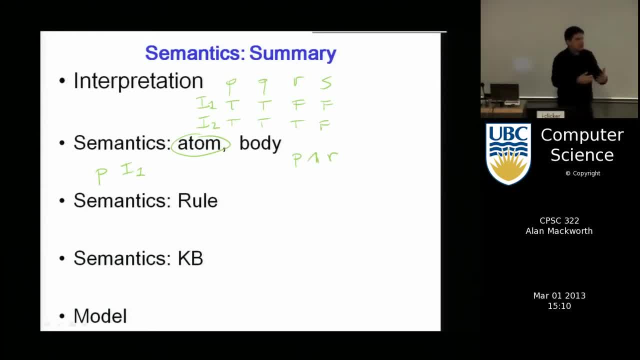 Remember we, we saw the semantic. the semantic of the end of the conjunction is true only if both are true. So this one is true in N interpretation of the two. Which interpretation is true? I2. Okay, Because both are true. 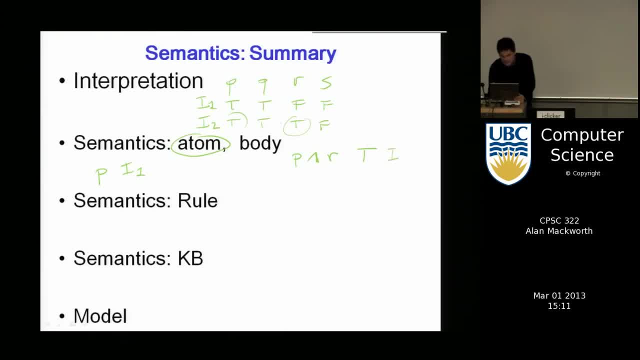 Okay, Why do you? if it's false in interpretation? Why? Why Okay? So if somebody is showing you a body and is telling you: is this true or false, you cannot answer it unless somebody is telling you with respect to a particular interpretation. 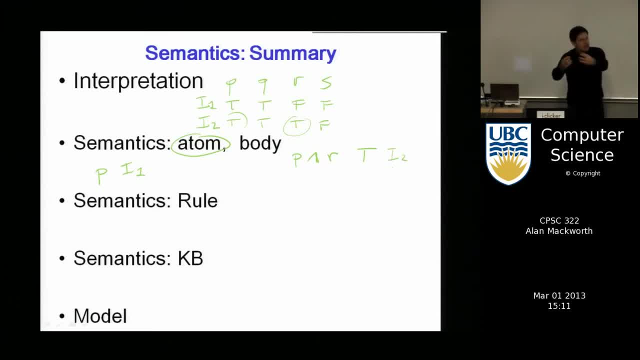 Given the state of the world. that's why the semantic Given a connect, a description of what is true and false in the world. you can say whether a certain logical statement is true or false. Okay, So now that we have the atom, the semantics for atom and body, 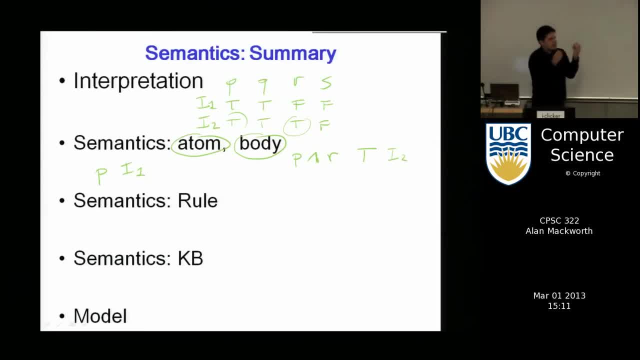 Because the rule, remember, is a body, imply an atom. We can now specify the semantics of the, of the rule. Okay, Of the rule, like of the form, let's say E, U and S. Remember what is the semantic for? for the rule. 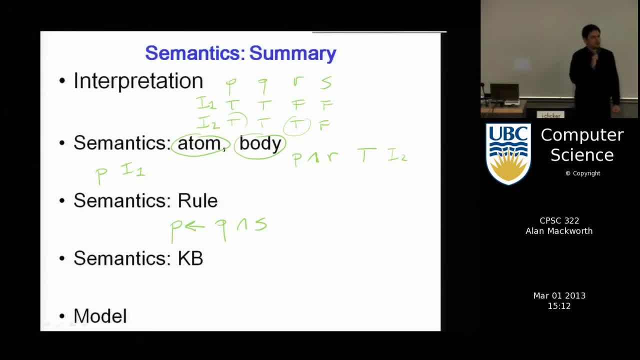 The rule is true unless always true unless this is true, but the S is false. Okay, So now you can apply that to an interpretation. Let's say: in E, in I1, what is the body? Q and S Is false. 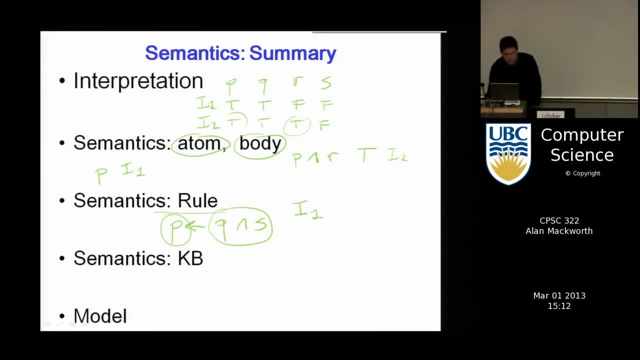 So you already know that this rule is true. So when, when the antecedent is false, it doesn't matter what is the, the consequence? Let's say, for I, I2, Q and S is true, And Q and S is true. 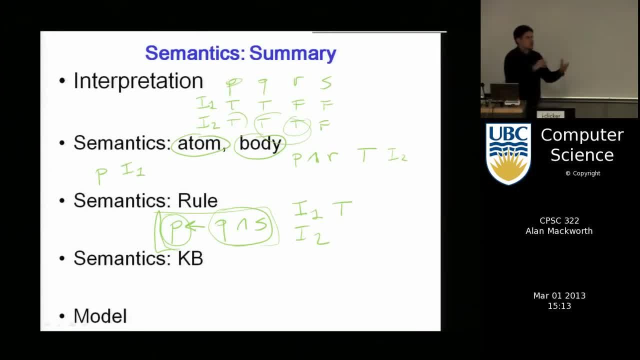 And P is true, So, true, true, it's okay, Thank you, Which one? Yeah, Q is true, S is false, So this is false. So the the rule is true, Because the only case in which the the rule is false is when the antecedent is true and 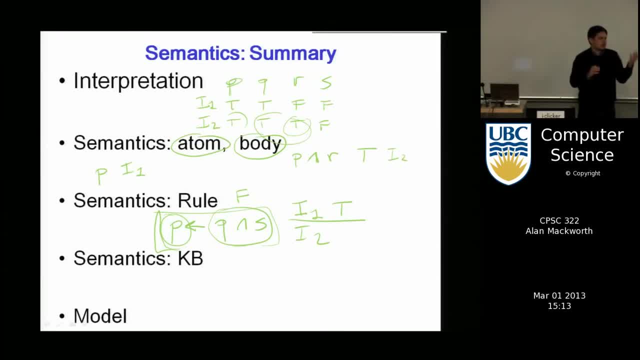 the consequence is false. So if you, if the antecedent is false, you don't even need to check whether the the the consequence is true or false. So in both interpretations is the rule is. So what would be an interpretation in which this rule would be false? 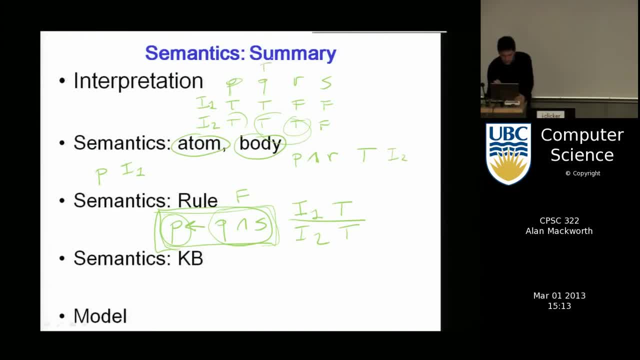 It would be an interpretation in which you have Q true, S true and P false. Okay, And R doesn't matter, Okay, Because in that case you have the antecedent is true and the consequence is false. Okay, So let's call it is I3.. 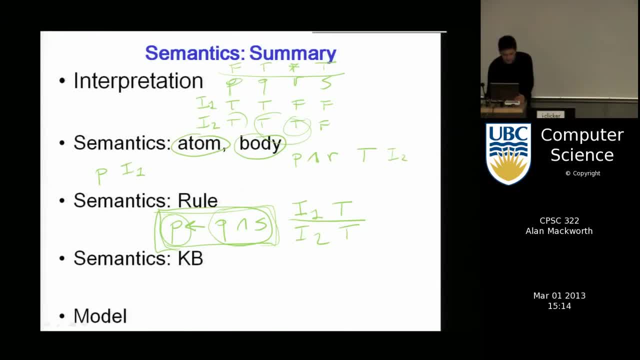 So this rule in I3 is false, Okay, Because the antecedent is true, but the consequence is false, Okay, So now you see there is a composition. That's what logics they? they do this, this kind of thing. 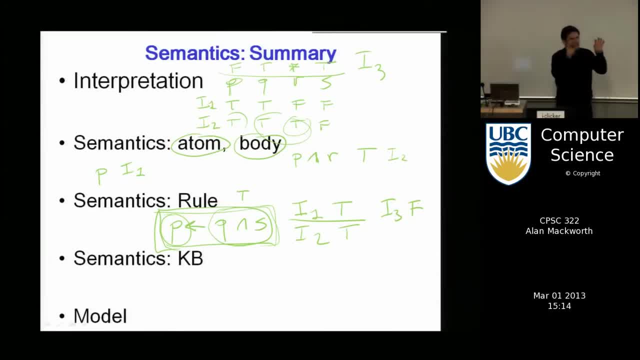 Okay, They do this, this semantic composition. We start from the building block, the atom. the body is built by atoms, the rule is built by bodies and atoms. Now, what about the semantics of a knowledge base? What is a knowledge base? 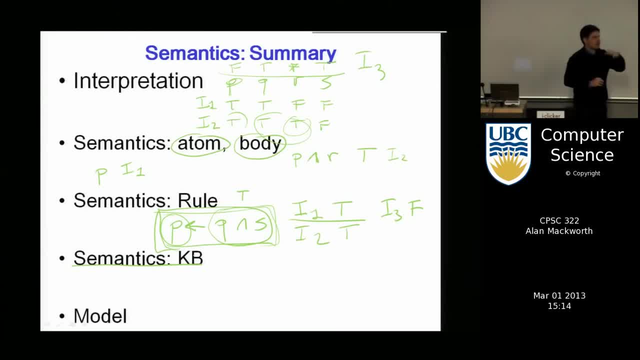 It's just a set of definite clauses that can be atoms or rules. When a knowledge base is true in an interpretation, well, when all the clauses are true in that interpretation, Okay, we have the knowledge base P and Q multiplied by S. so this is like two definite clauses. 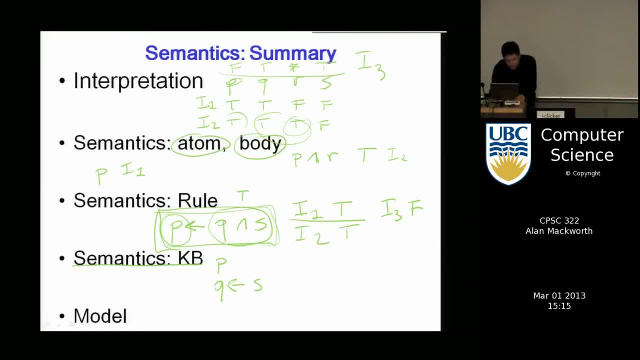 one atom and one rule. to check whether this is true in interpretation one. well, you need to check whether P is true, the first clause, which is ok, and the second clause, whether the rule is true. you check: S is false, so the rule is for sure, true. so the knowledge base is knowledge base. 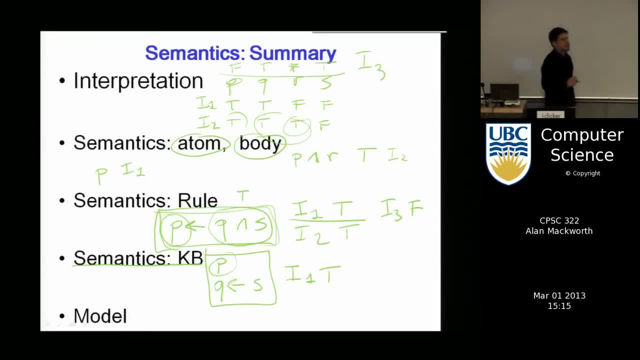 a set of clauses is true in interpretation one. so mechanically we can give a knowledge base and an interpretation to answer the question whether the knowledge base is true in that interpretation. ok, so that's the first step of the semantics. ok, for each possible form in your logic. 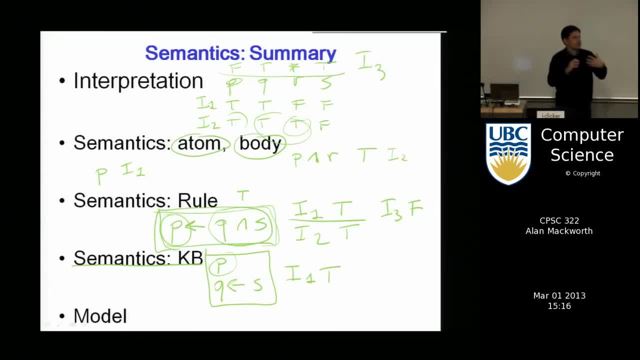 you need to be able to automatically compute to automatically say whether S is true in a given interpretation. ok, so do you remember what a model is? a model of a knowledge base. so you define a model of P is what it's: an interpretation in which the knowledge base is true. 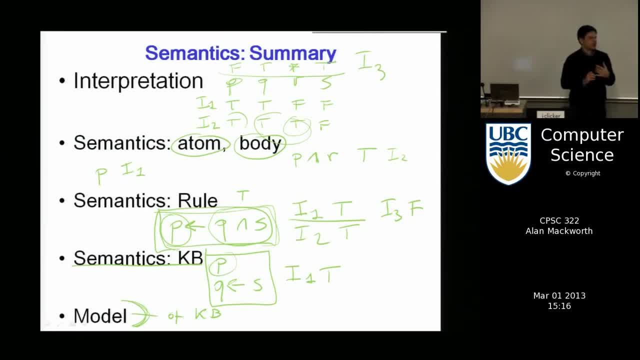 ok, so every interpretation in which a knowledge base is true, it's a model for that knowledge base and if you want to think semantically, it means like, given what I know, that is your knowledge base- a bunch of formulas. in our case it's very simple: atoms and rules. 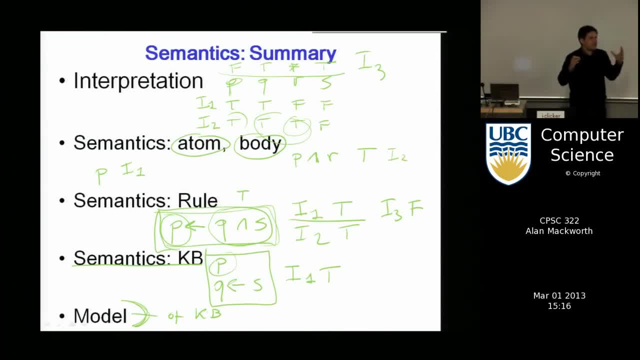 all the models are all the interpretations, all the possible words that are consistent with what I know. ok, in which what I know is true. ok, so let's look at an example of models. so if I give you a knowledge base and I ask you, I find the models. 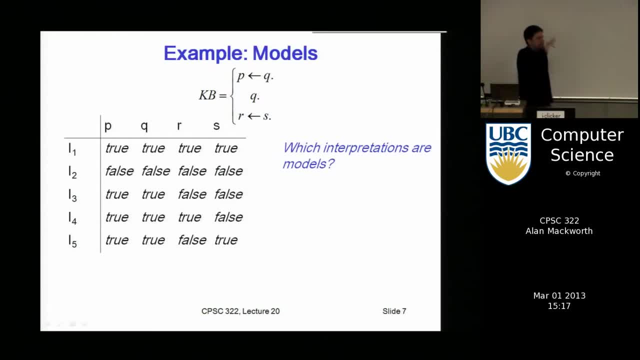 what do you need to do? you need to think of all the possible interpretations. are these all the possible interpretations for this knowledge base? how many propositions? how many propositions? you have one, two, three, four. so how many interpretations there are. 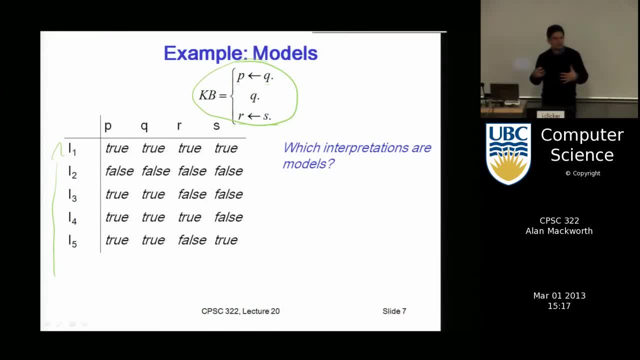 your environment can be in two to the fourth possible states. so there are two to the fourth interpretations. so these are not all of them. ok, which one are models? how do you check? I mean, you can go through each of them. is this a model? 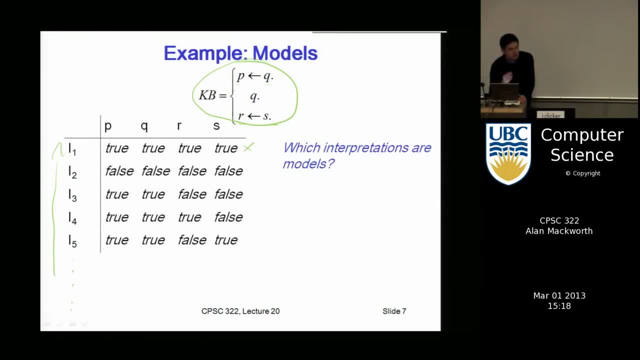 what do you need to do? you need to check. you need to check for each clause in the knowledge base whether it's true in the interpretation. so in this case, they're all true, it's ok. they're all true because Q is true, it's ok. 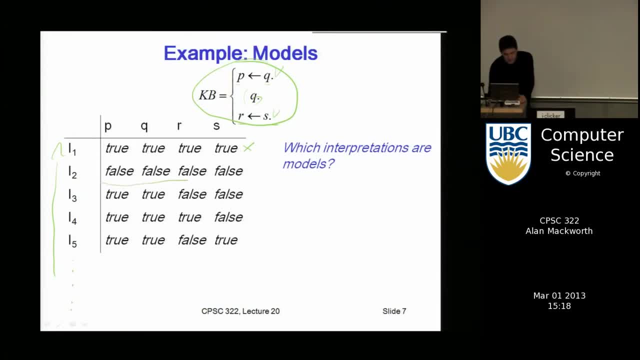 2 implies 2, it's ok. 2 implies 2, it's ok in this one. well, Q is false. so you already find a clause, definite clause, in your knowledge base. that is not satisfied, so sorry, let's use this. so this is a model. this is not a model. 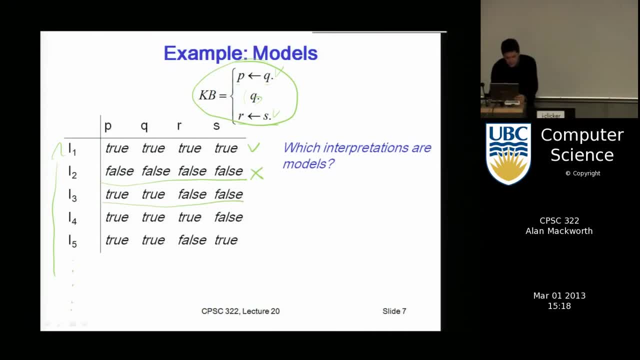 what about this one? check Q, it's ok. then Q implies P, Q is true, P is true, so that's ok. S implies R: it's false, R is false, so that's ok, ok, ok, so, model, let's do this, this other one, so Q is true. 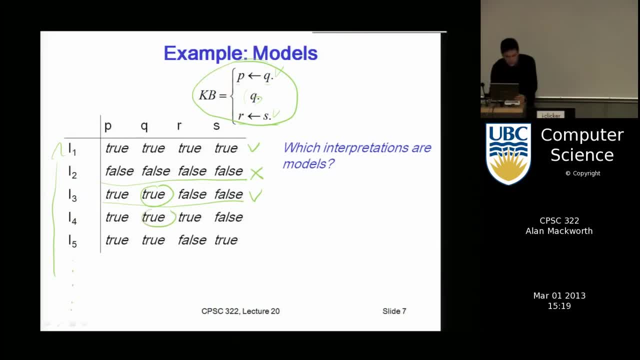 so that's ok. P implies Q. they're both true, so it's ok. S implies R, false implies true. is it ok? yeah, this is not ok, because it's true implies false. so this is not. this rule is not true in interpretation 5. so interpretation 5 cannot be a model. 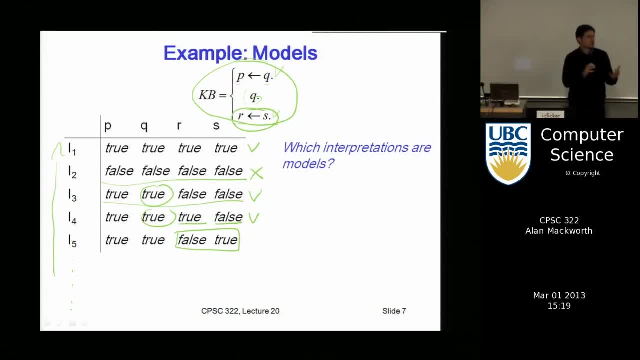 as long as one clause is not true in the knowledge base, as long as one clause is not true in the interpretation, that interpretation cannot be a model. ok, so why do we care about these models? as I told you, they are the interpretations that are consistent with our knowledge base. 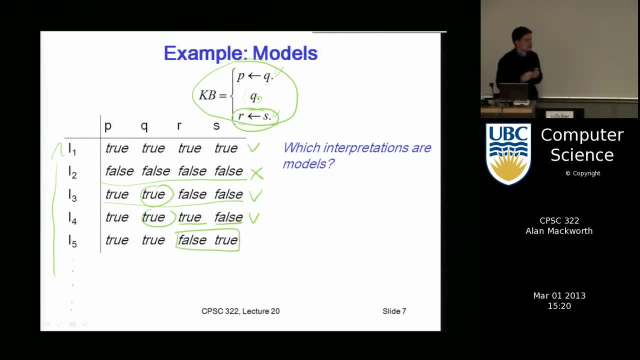 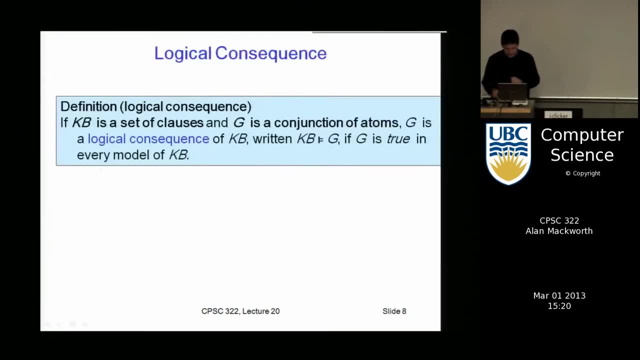 but what can we? ok? ok, you know that these are all the models where this is a important definition. it's a key definition in logic that if you have a knowledge base and you, you know where are the models, well, you would like to know what else is true in all these models. 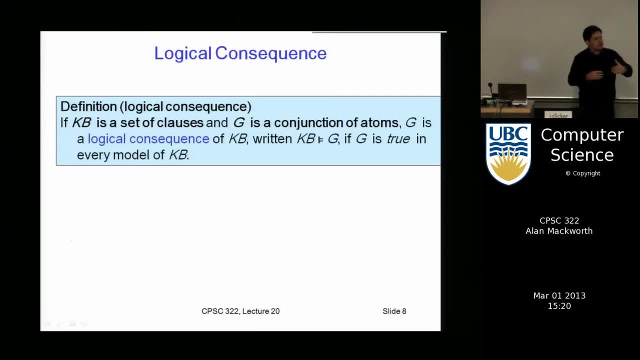 ok, it's something that, going beyond what you already know, what is logically entailed? well, it's what is true in all the models. it's including what you already know, but what else is true? so that's the idea of being logically entailed- follow logically from a knowledge base. 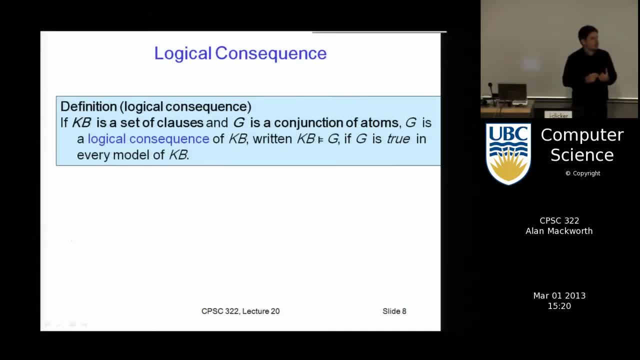 is what is true in all the models for the, for that knowledge base. ok, and that's what we would like to be able to infer, to deduct from, from what we already know. what else is must be true given what we know? ok, so that's the definition. 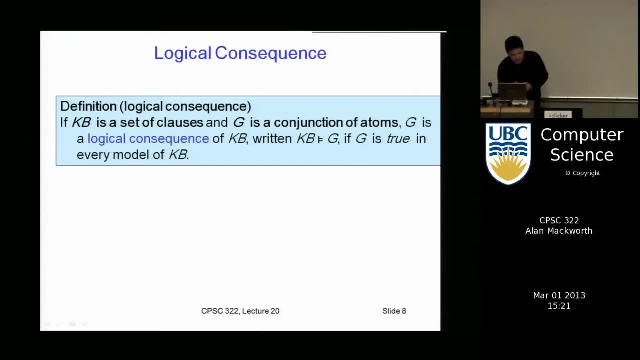 of of logical consequence. so, given a knowledge base, g are conjunctions of atoms, so it can be like p, q, g is a logical consequence. if it's true, in all the models, in every models of the knowledge base, and that's how we write it. ok, we're going to see an example. 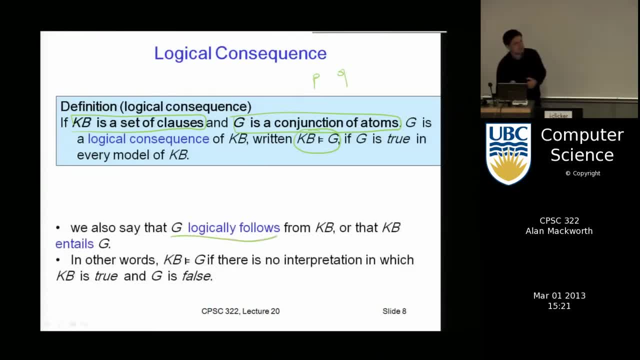 of that. so you can say: g logically follows. again, g logically follows from a knowledge base. if it's true in all the models, and just to get you to the kind of twist of words that you use when you think in like logical terms, you can also say that: 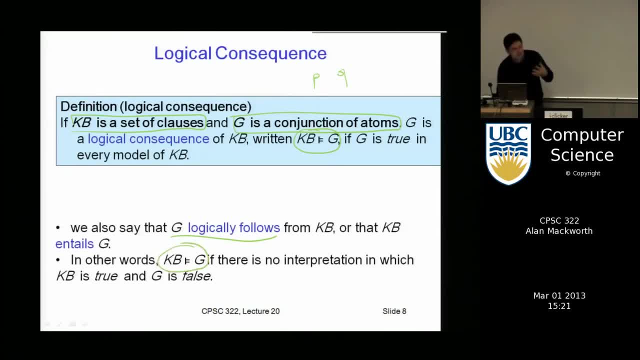 a knowledge base logically entails a set of atoms. an atom or a set of atoms. if there is no interpretation in which the kb is true and g is false, ok, so what is this interpretation in which kb is true? model? so you're saying, if there is no model? 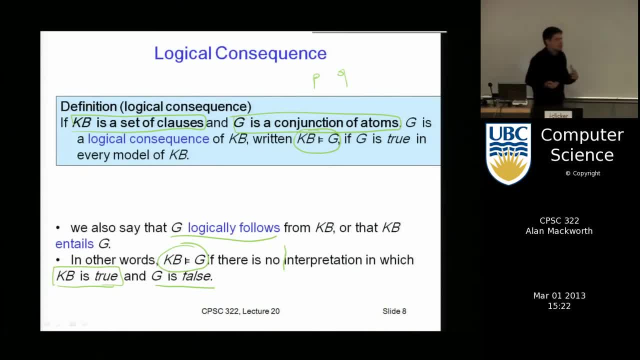 in that model g is false. why? because, by definition, you're saying that something is logically entailed if it's true in all the models, so that there is no model for the knowledge base in which which g can be false. ok, so let's see an example. 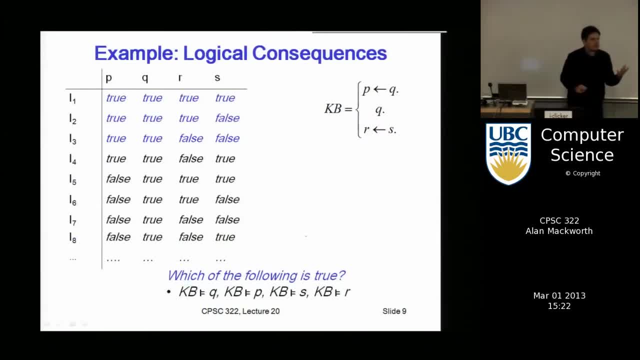 of what is the logical consequence of a knowledge base. so you have the knowledge base. I'm telling you. these are the models. what is this? it's a subset of the interpretation. so why do you know that, even for this knowledge base, there are two in the fourth interpretation? 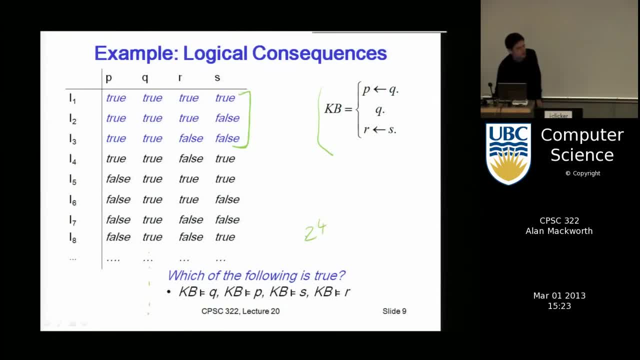 there are eight more here. why do you know that? there are no models. you see, in all these q is true, so in all the other ones q has to be false. but if q is false, one clause in the knowledge base is true. the knowledge base is false. 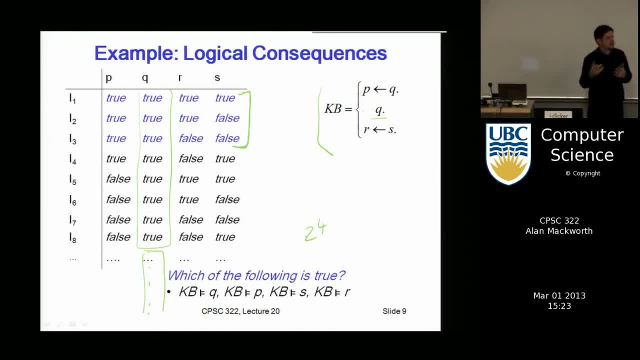 so those interpretations, in those interpretations, the knowledge base cannot be true. ok, so you can just not even consider that. ok, so these are models. what is logically entailed by this knowledge base? well, I just gave you the definition. it's everything that is true in all the models. 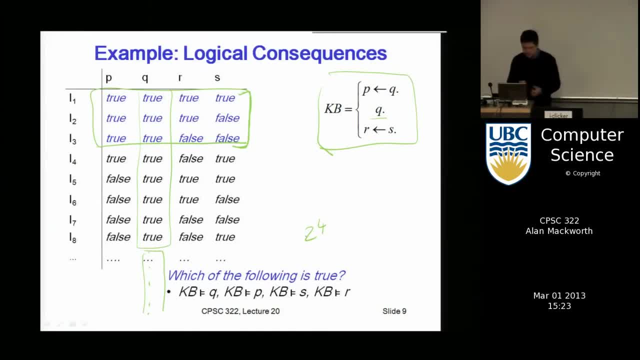 so what is true in all the models? q? r is not s is not so. if you are asking whether the kb is the way to us, is the kb logically entailing q? yes, because it's true in all the models. is the kb logically entailing p? 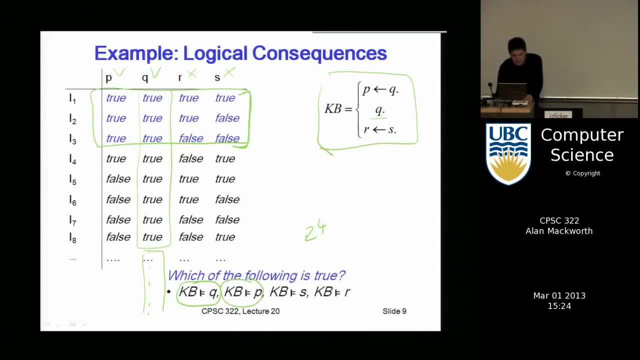 yes, is the kb logically entailing s? no, so when you write in the result what the bottom is and r, is not true in all the models. yup, just two questions. a notation: you said that the kb, and between the proposition. what does that sign actually mean? 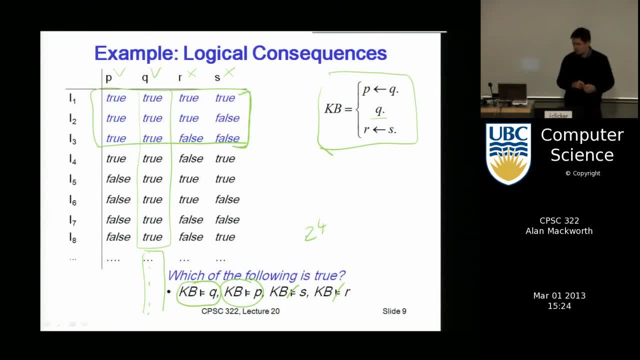 it's a pretty time consuming which sign between the kb and the proposition. so kb? so it's asking. it's saying kb logically entailed or q is logically entailed by the kb. and what was the symbol? the symbol, oh ok, that's the notation. 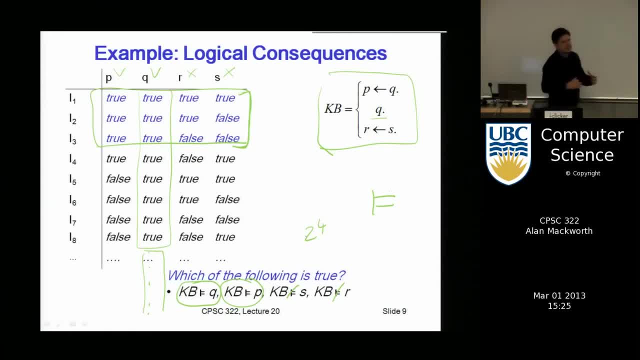 the logical notation in logics. if you want to say that the knowledge base is entailing, is logically entailing something, it can be a formula. in our case, it's an atom or a set of atoms. that's the symbol that we use and you're gonna see why. 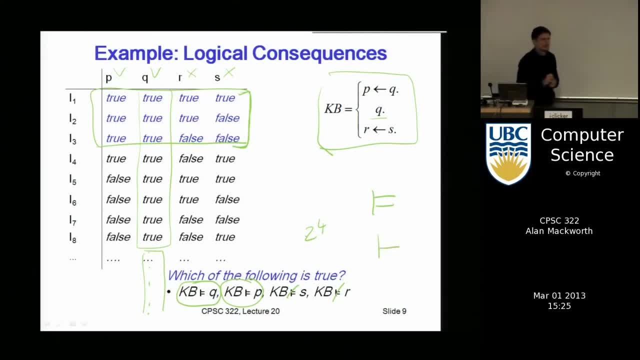 it's different from this symbol. that means you can prove by using a proof procedure and if you, if you vary, the meaning is: this is not logically entailed by by the knowledge base. yup, in this case, can you say? s implies p um. p is what. 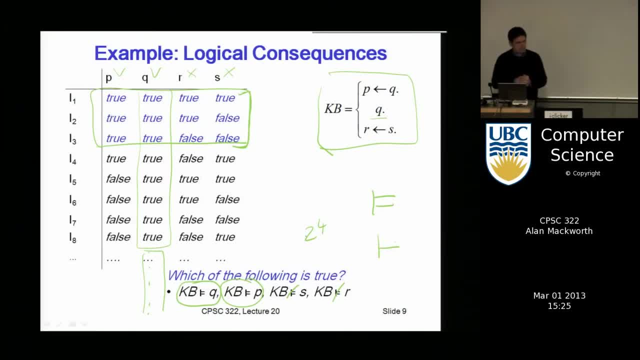 which um logically follows from this? um, we are not. we are just trying to to verify whether an atom or a set of atoms are logically entailed. so we don't have a, it is so. you are just saying. you said because it's that formula is true. 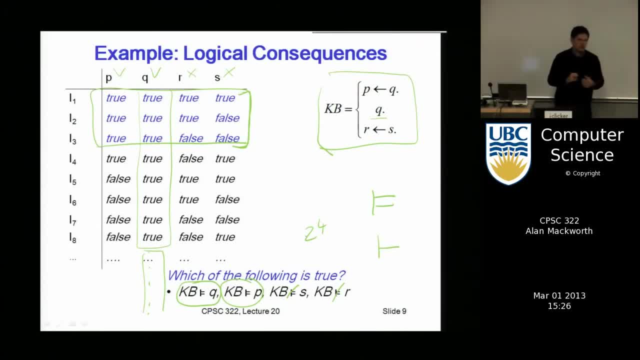 in all the models. yeah, if you added more power, you should be able to realize that. but you are focusing on proving, uh, and defining whether an atom or a set of atoms is logically entailed. yeah, that's a good point. yeah, so you talked about the distinction there. 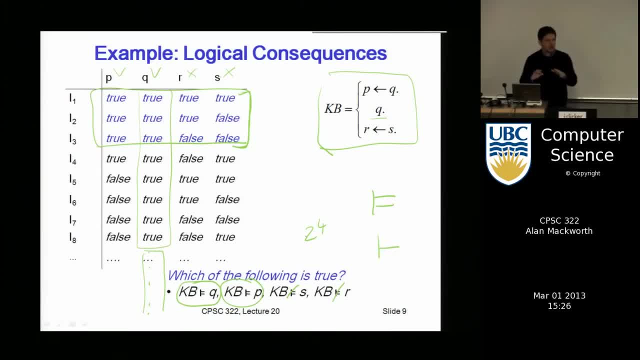 between the two symbols, one for logical consequence and the other for provability. yeah, but I've worked on that, so like that presumably has to do between, to do with the distinction between syntax and semantics. yes, and how do you count if your theory of truth and your theory of provability? 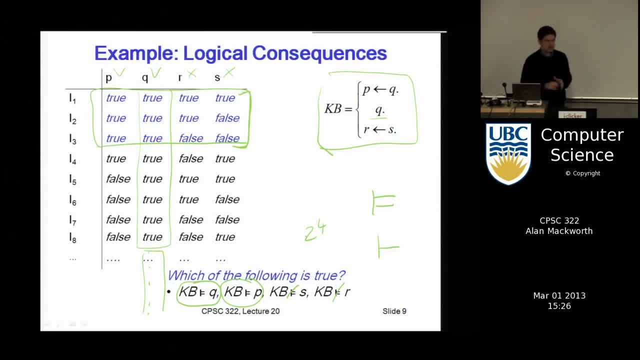 have to be different. yeah, we are moving now in that, exactly in that direction. so now that we kind of know what I mean, we know what is an interpretation, what a knowledge base, what it means for a knowledge base to be true in interpretation, what is the model. 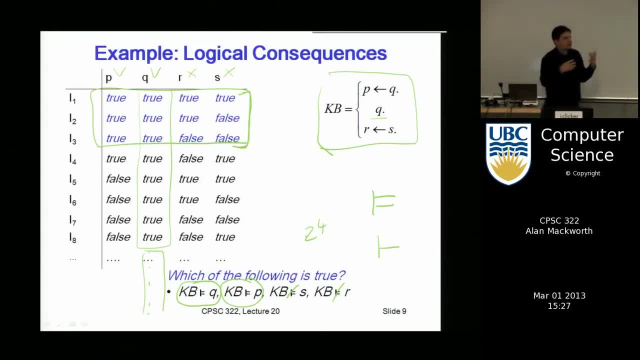 logically entailed. we said that, well, it would be great, given a knowledge base, to know what is also logically entailed by the knowledge base, because we know that that must be true, but we don't know even what we know. so how can we derive that? ok, 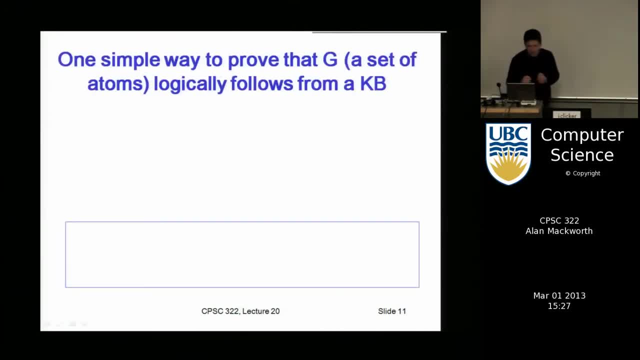 what is a simple way to prove that a set of atoms- this is our question. just, we are working on a set of atoms- follows from a knowledge base. if you had to write a problem, I give you a knowledge base. you can give all the possible interpretations for each of these. 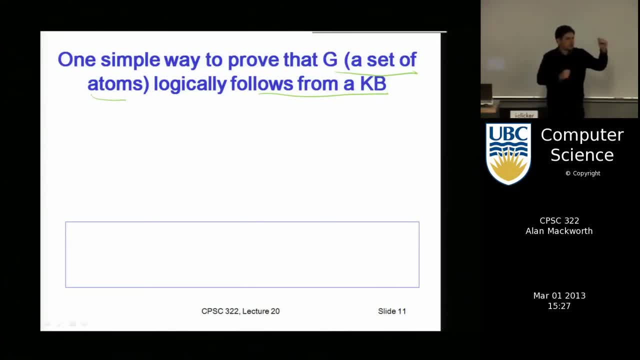 for each of them. you can check whether it is a model or not, and you select the model and you check in it for whether what is true in all the models and that is logically entailed. ok, so are we done? just a bunch of loops, are we done? 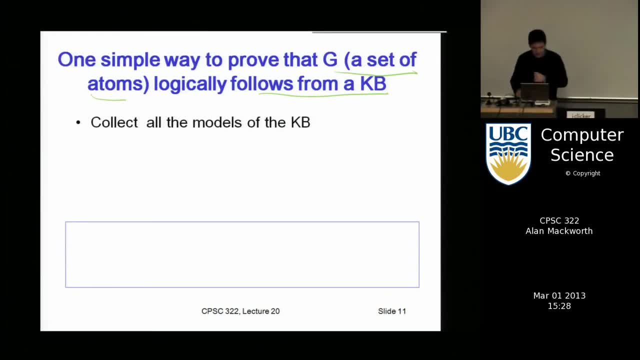 ok, select all the models, verify the history of all those models and we know whether G is logically entailed or not. ok, or you want to say something about this, but that's not for now. it might be a problem, but that's the problem. ok, if you describe a domain. 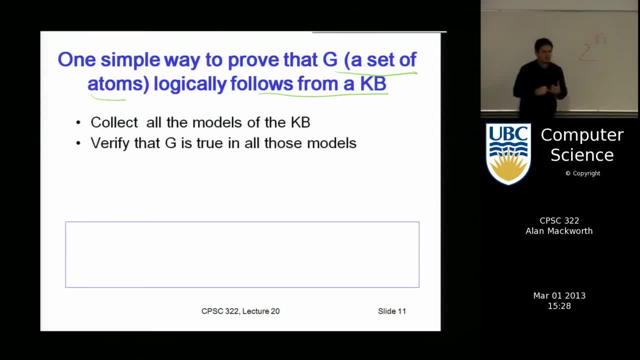 where you have ten thousands propositions and you want to go through the ten thousand interpretations, and so the whole development of logics and practical way to perform reasoning is to be able to infer what is logically entailed without going to all the interpretation and finding out what are the models. 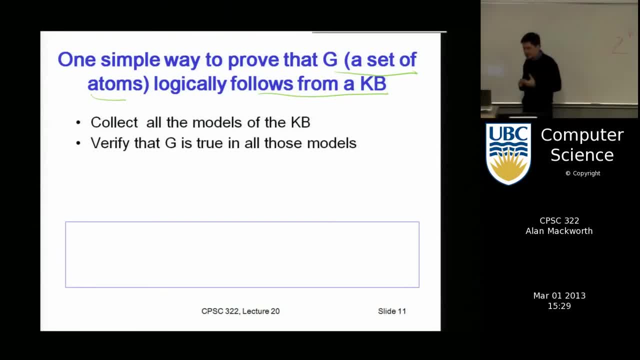 and what is true in all the models. ok, so that's the the key idea of of the proof procedure, something that you can apply syntactically to the knowledge base and somehow is correctly telling you whether something is logically entailed or not, without going through this semantic. 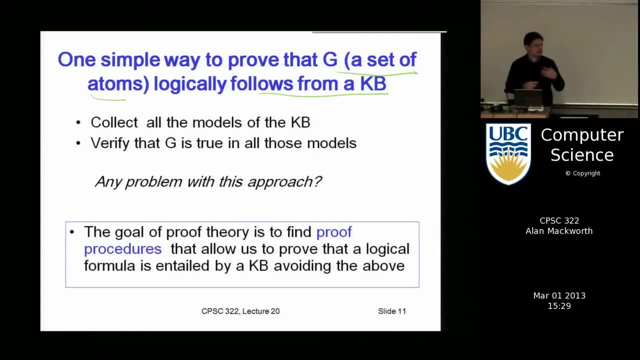 which is this process of going through the interpretation, verifying whether the models are true interpretation or not. ok, so finding a. yeah, is there another algorithm to find the set in logit? ok, we are going to see now. we are going to see now a kind of a. 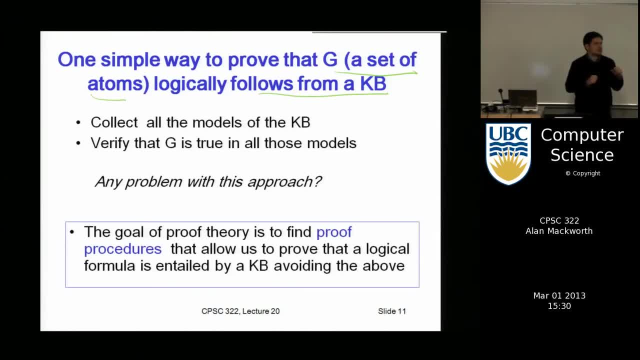 dumb procedure, proof procedure, but it it can. it can compute what is logically entailed and what is not logically entailed, and then in next week you are going to see a procedure that is smarter and more efficient. but now, before we look at this proof procedure, there is something that is. 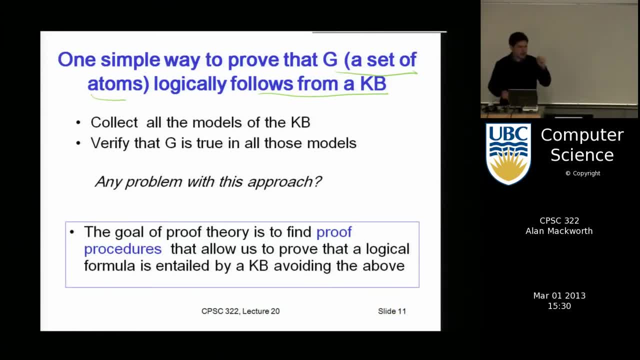 kind of the next level of complexity in logic. if I give you a proof procedure, you need to prove something about the proof procedure before you can use it. so that's why logic becomes a little bit confusing and challenging. but luckily we are working on a very simple logic. 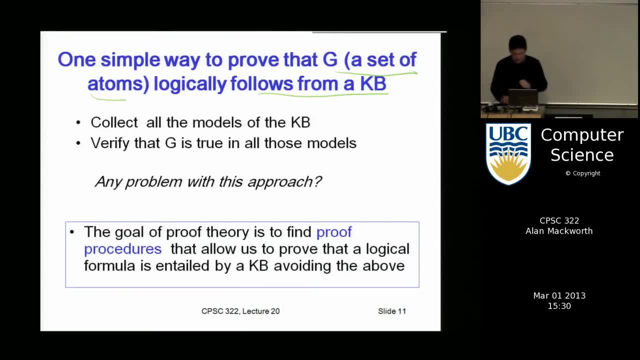 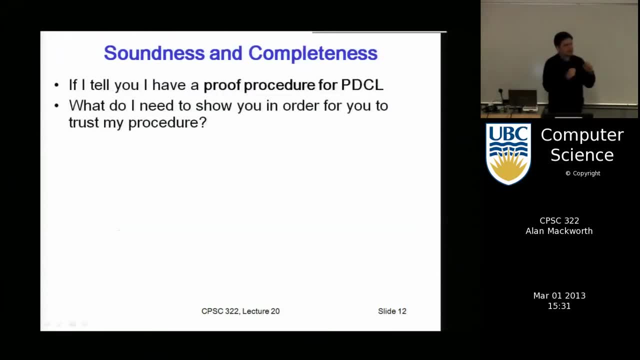 so what we need to prove is going to be relatively simple. ok, so let's say, let's say that I tell you. ok, I have this proof procedure. it's kind of syntactically manipulating the knowledge base and it's telling you, uh, whether something is logically entailed or not. 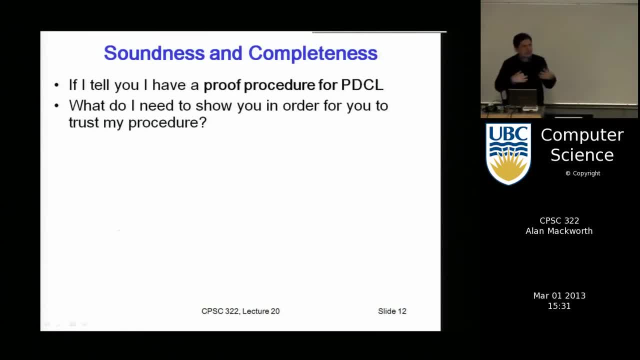 can derive. can derive what you need. are you going to trust this procedure? how do you know that this procedure is always going to tell you it's always going to derive only what is logically entailed and it's not going to derive what is not logically entailed? 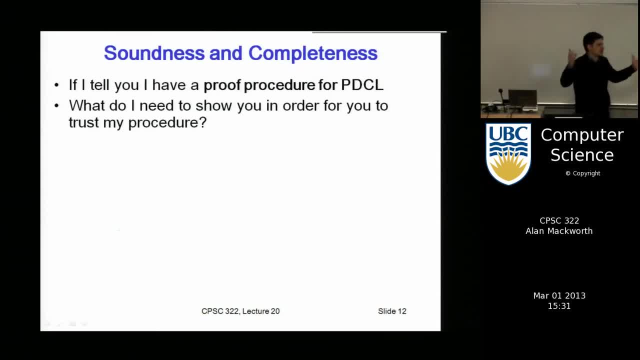 we are talking about like billions and billions and billions of possible interpretations, and so if you are simplifying a problem by doing something syntactically, you need to show something about your proof procedure. you need to prove something and the two properties that you need to prove. 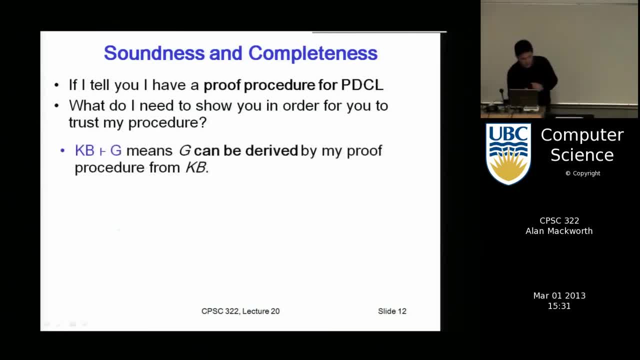 using this terminology. so we say that you can derive G with your proof procedure from a knowledge base with this symbol, and we already saw the symbol for saying that G, this set of atoms, is logically entailed. it's true in all the models. you need to prove that these two sets are the same. 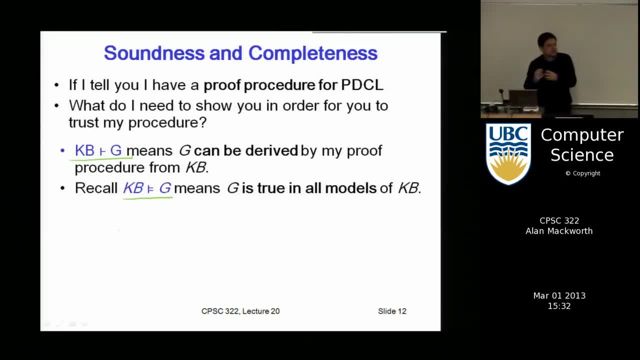 whatever can be derived is logically entailed. and whatever is logically entailed can be derived by your proof procedure. so this is what is called in logic, to prove that, the soundness of a proof procedure. so you want to show that whenever your proof procedure you are going to see now 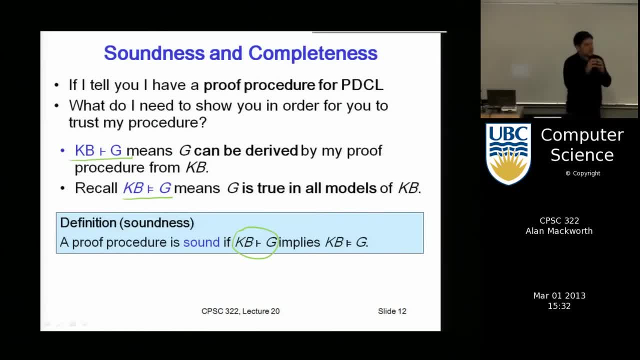 a very simple proof procedure. it's telling you G I can derive this set G. well, you need to prove that, that this set G is logically entailed- it's true- in all the models of your knowledge base. and then you need to prove also the other way. 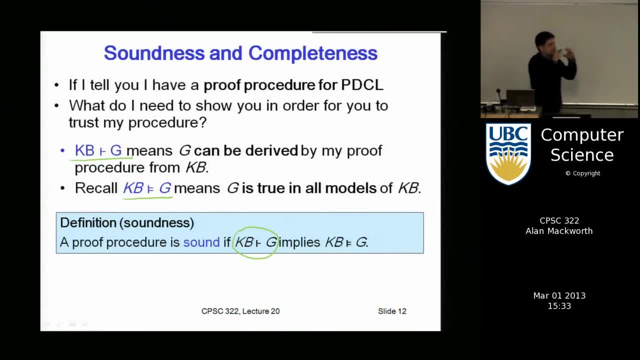 that everything that is logically entailed. so if an atom or a set of atoms is logically entailed- it's true in all the models of a knowledge base- it can be derived by your proof procedure. so that is true in all the models of a proof procedure. 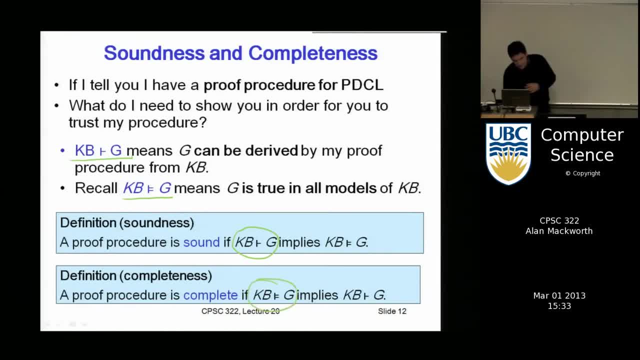 so we are saying that if set of atoms or an atom is logically entailed, well, you are going to be able to prove with your proof procedure. your proof procedure is going to say, yes, this is, this is provable. ok, so we are now going to look at the proof procedure. 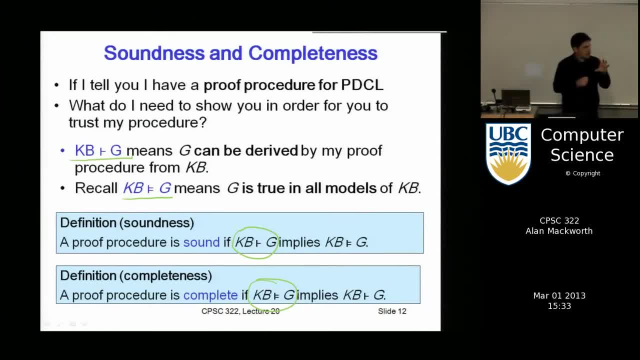 for, for definite clause logic, propositional logic, which is going to be syntactic manipulation of the knowledge base, of the knowledge base, and then we are going to at least cover the proof of the soundness of this proof procedure. ok, this is a tricky concept, but when you see it applied to a real 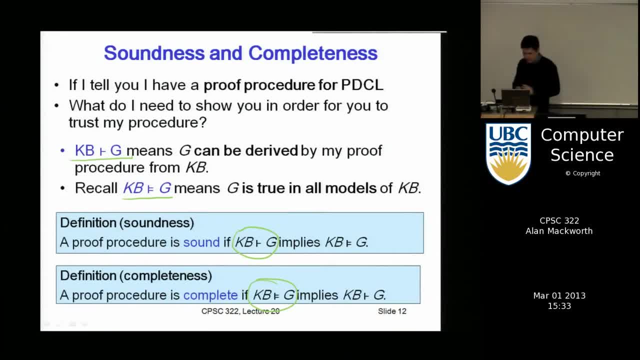 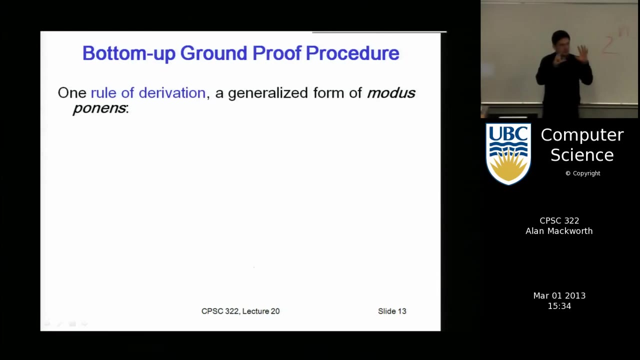 a real proof procedure. it's going to be, it's going to be clear, and that's why we want a logic that is super simple. so these proofs of soundness, completeness, their complexity grows with the complexity of your logic, ok, ok, so let's start describing the proof procedure. 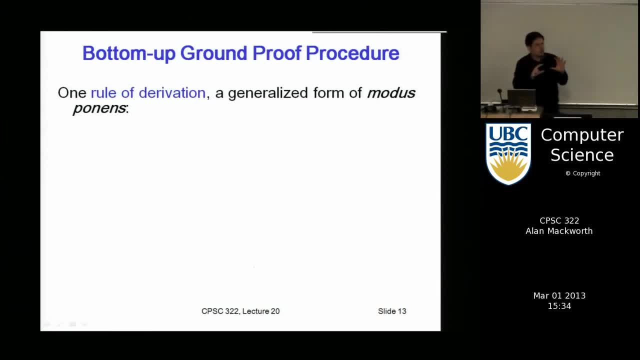 it's using only one simple syntactic manipulation of the knowledge base and it's the generalized form of modus ponens. so this comes from like 2000 years ago. if you add the implication pq and q, so let's say that this is your knowledge base. 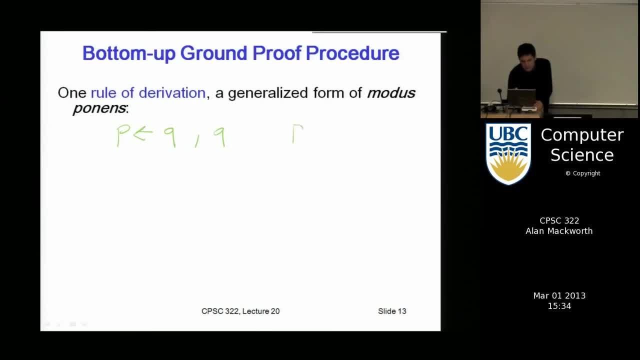 you can derive just p. ok, so you can add p to your knowledge base. syntactic: whenever you have a clause with two atoms and one is already in your knowledge base- the antecedent- you can add the consequent to your knowledge base. so we generalize this by saying that: 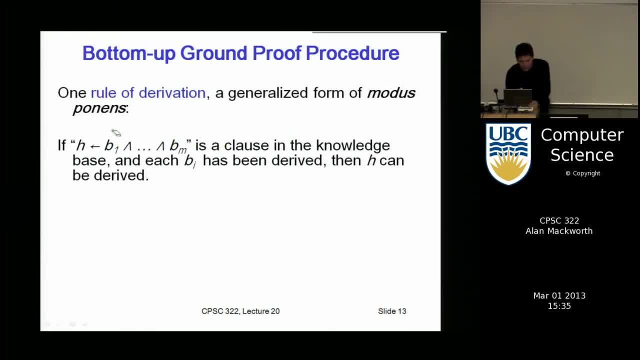 if you have a clause in your knowledge base like this: so this is the body and you have been already able to derive all the atoms in the body. derive means nothing semantically, like syntactically. you have been able to derive those, then you can derive h. 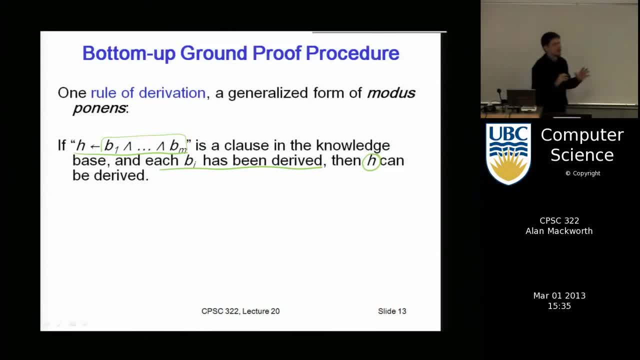 ok, so this is the only rule that we are going to use, and I'm going to show you how you can use it systematically to be able to decide whether a set of atoms can be proved or not. ok, you can see this forward chaining on this clause. 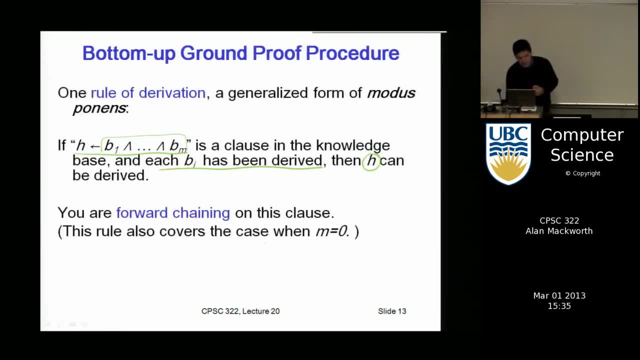 and also this covers the case when n is equal to zero. ok, so what does it mean that n is equal to zero? I mentioned last time, if you have p in your knowledge base, you can think of p. you can think of p as like the clause with no antecedent. 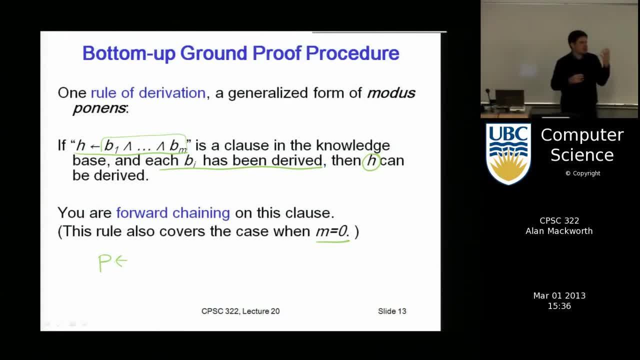 so this is saying that if you have p in your knowledge base, p can be derived by this rule, by this rule. ok, but you don't need anything to be already derivable to be able to derive the hat of this, ok, so let's look at the. 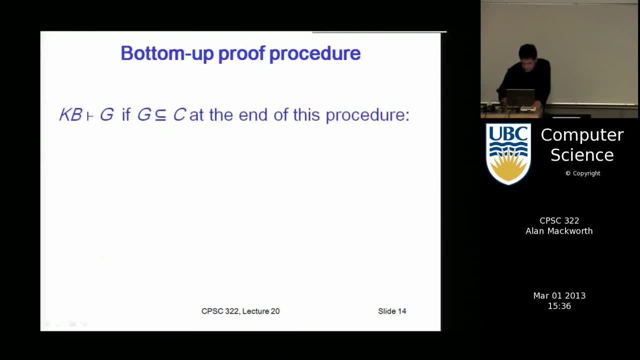 the full proof procedure. so we apply the proof procedure in a way that we are building a set and then at the end, when we have this set, we say that our g set- that we want to verify whether it can be derived or not- is derivable only if it's the subset of the set that we have created. 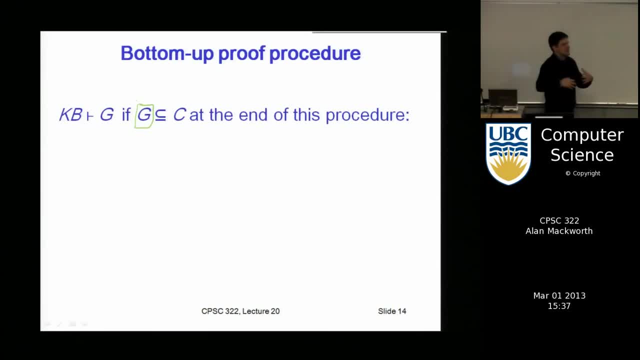 ok, so the proof procedure is just creating set c and then, at the end, to see whether g can be derived, we just check whether it's the subset of c. so how we create this, this set c, ok, we start with the empty set and then we repeat this. 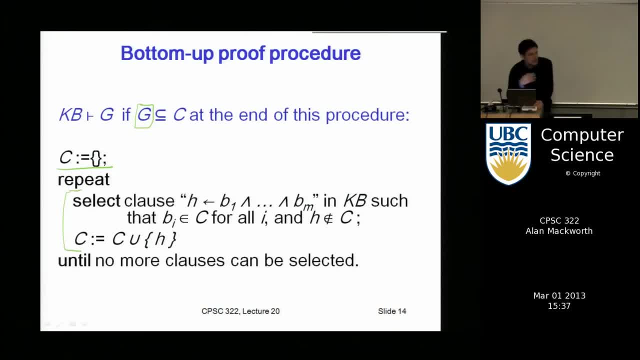 this step as long as, as long as it's possible to to repeat this, set this step. ok, we select a clause from the knowledge base and if all the antecedents, the elements of the body, are already in c, we can add h to c. ok, so we need to condition that all the elements are already in c and 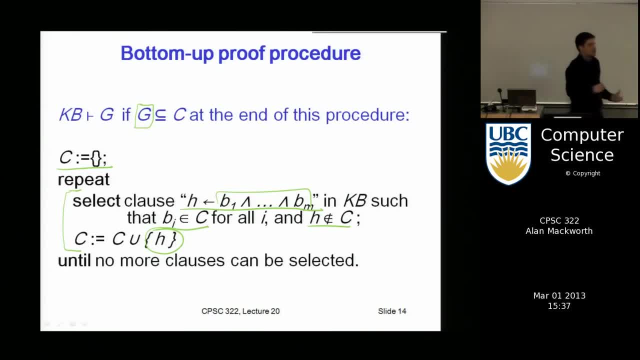 that h is not in c, the head is not already in c. ok, so we keep applying this as long as this is possible. we are creating this set c, and then we just need to verify whether g is the subset of c and then, if that's the case, 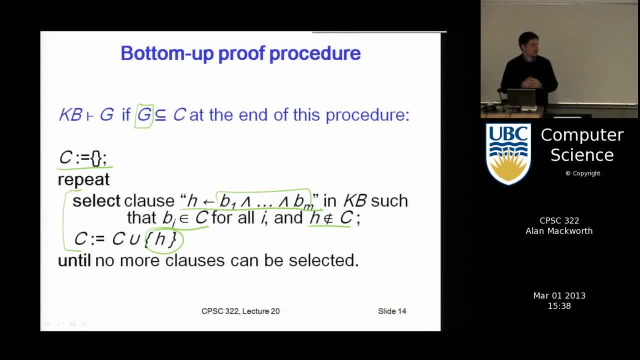 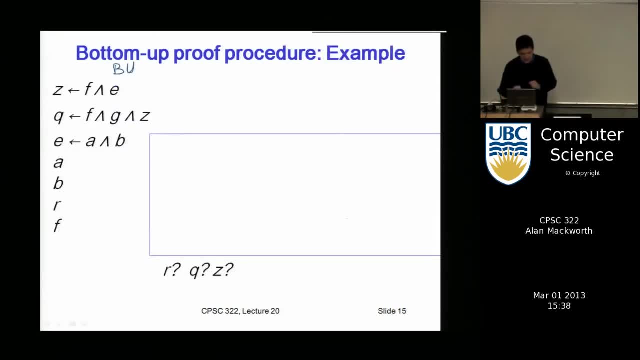 we say we can derive, we can derive g. ok, let's see an example. that should make everything super clear. so, given a knowledge base, we start with c empty. then we select a clause for which the d, i are already in c and h is not in c. 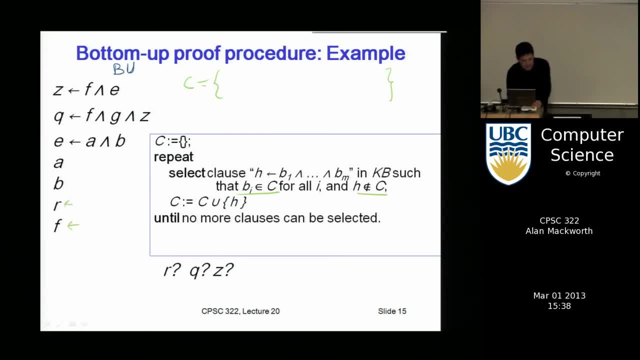 remember. this can be interpreted as clauses without the antecedents. so we can add f to c, we can add r, we can add b, we can add a. ok, these are clauses in the knowledge base for which the antecedents are already in c, but the descendants are already in c. 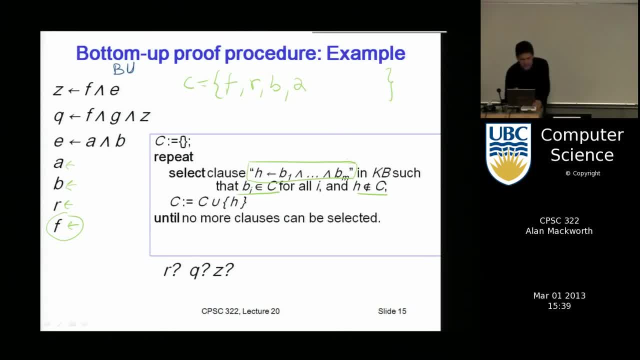 so we can do it. so now, what else? we can add? this clause? the antecedents are already in c, so we can add e. ok, what about this clause? so once we have added a clause, obviously we cannot re-add it, because h is in c. so what about this clause? 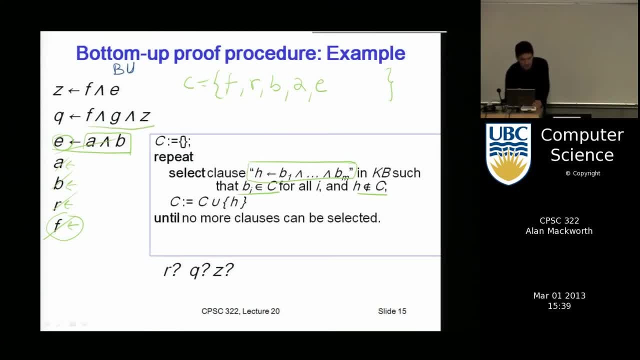 can we add it? can we? can we fire? can we add h when we check? f is in c, g is in c, but z is not. so this cannot be fired. no, g is not. you are right. so this is not. what about this? clause f and e? 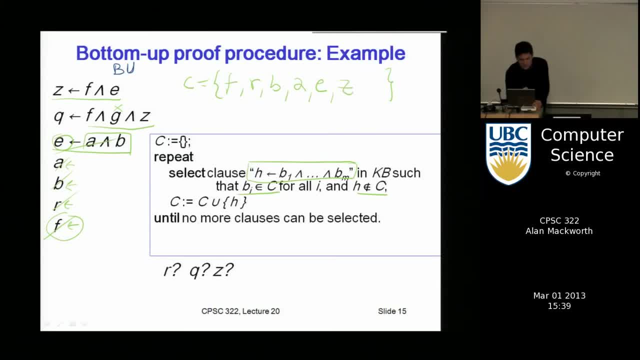 f and e. yes, so we can add z. so now we will check this one. but because g is not added, we cannot add q. ok, so the key point is that what we are doing is just syntactic manipulation of the knowledge base. we start from the set. 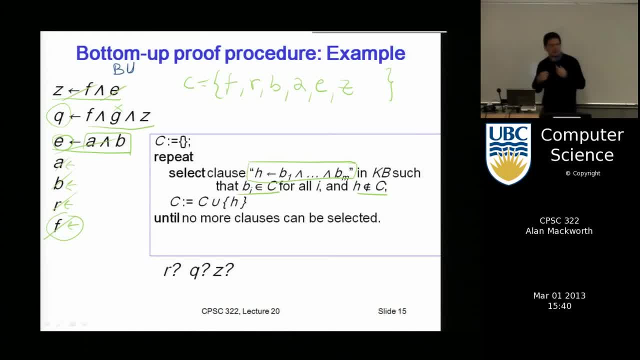 we add stuff, if we add new atoms to this set, if this condition is satisfied, when we cannot add anything else, we add this c. and now you wonder, it's r, q and b are derived from the, from the knowledge base. you just need to check whether r is in c. 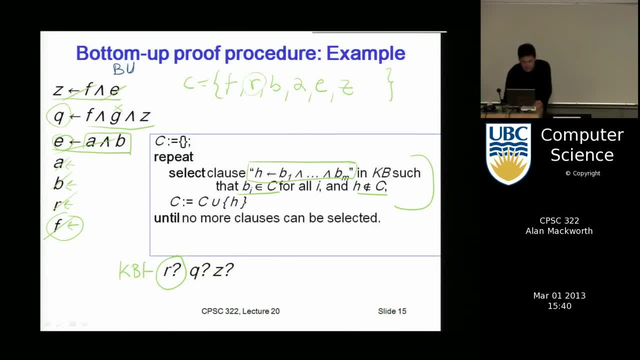 yes, ok, what about q, a, b, q, not in c? so I give, I tell you: oh, this is the way to prove stuff in propositional definite clause, propositional logic go and and immediately you say: well, I'm not sure. is it true that whenever this says yes, 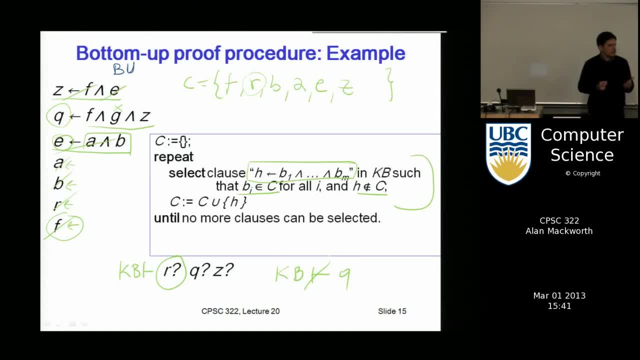 these are. this g is true in all the models of the knowledge base. I don't see why. so that's why you need to prove. given a proof procedure that someone is proposing, let's say that I'm just proposing this now, but now I need also to prove. 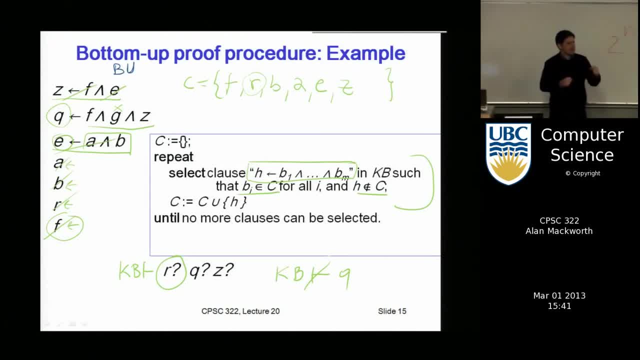 that it is the case that every time this proof procedure is telling you g can be derived, g is also logically entailed, and this is the sound, the soundness, and also you need to prove that everything, every time g, a set of atoms, is logically entailed. 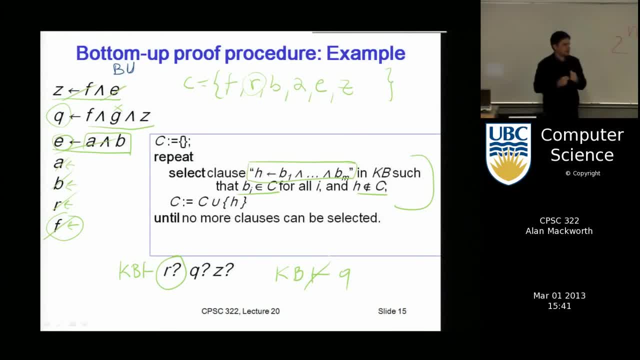 this procedure is going to derive ok, without these two proofs? well, you have. no, you cannot have trust that this is a usable, useful proof procedure. ok, so let's ok. I want to be sure that we do the soundness at least, so you can check with these questions. 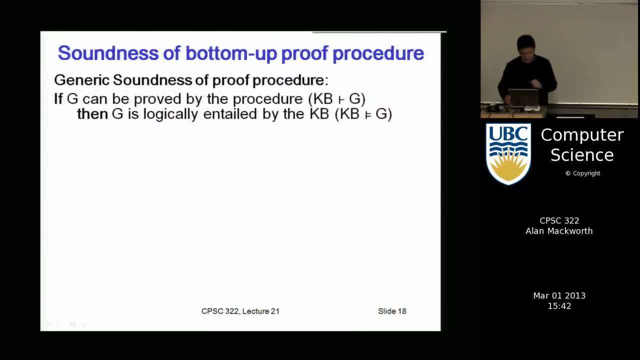 when you look at the slides. so let's focus on the, on proving at least the soundness of this proof procedure. is there any question on the proof procedure? you think you would be able, given a knowledge base, if I ask you: is this atom derivable or not? 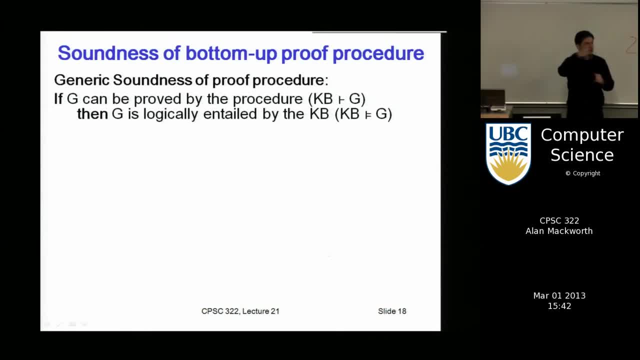 you just keep going through the machine and you create this c and then you check whether the your atom or your set of atoms is a subset. ok, now we want to prove that this procedure is sound. every time this procedure is saying yes, this set of atoms is actually logically entailed. 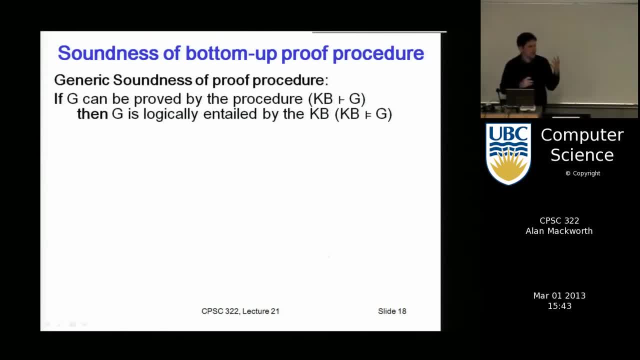 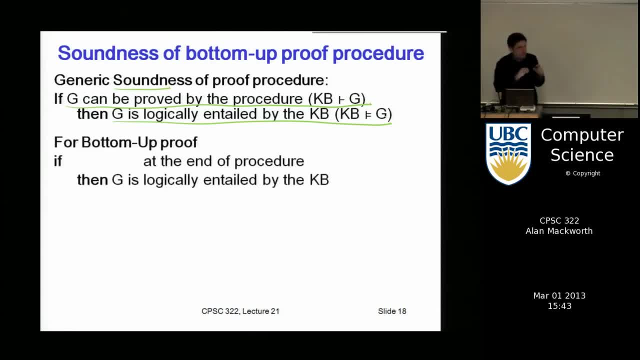 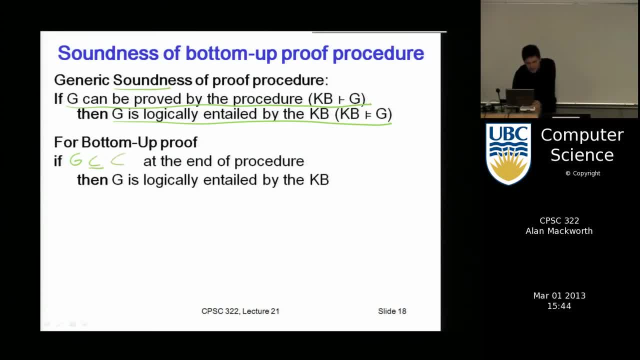 what we want to show is that if g is a subset of c- which is this set that is automatically by the proof procedure- then g is logically entailed. but this has to be true for any possible subset. ok, any subset of of of c means to be: 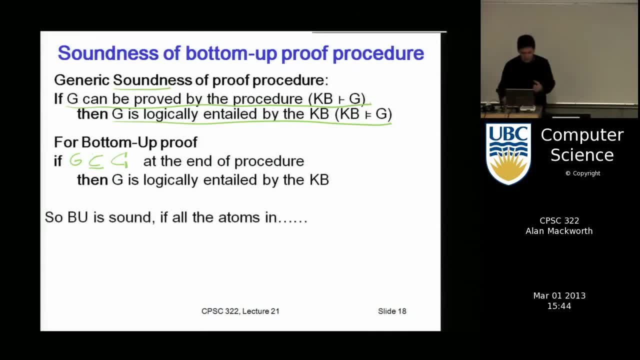 we want to prove that it is logically entailed. so what we actually need to prove that g is sound if all the atoms in c are one are logically entailed. that's what we are saying. we are saying that whenever a subset is is derivable, it has to be logically entailed. 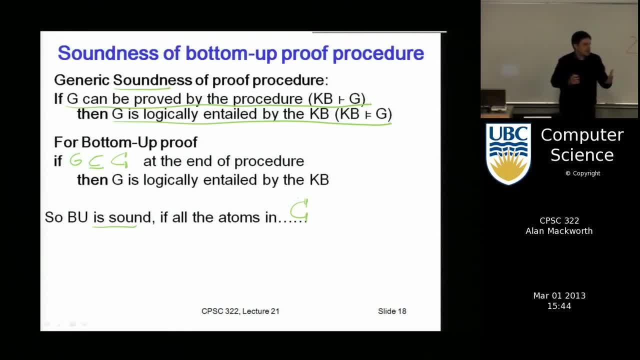 but it can be any subset including the whole set. ok, so all the elements in c, they have to be logically entailed. for our proof procedure to be sound, ok, and to be logically entailed, they must be true in all the models. ok, so now in a few minutes, 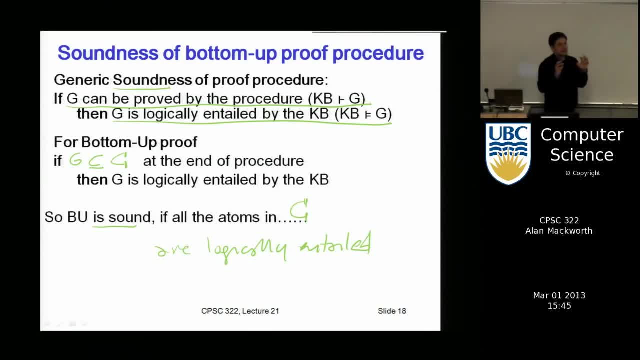 we are going to look at this proof which is combining. you are going to see how we combine syntax and semantics and I broke it down into steps and the first time is kind of puzzling, but then, if you go again, you might have time to go twice through it. 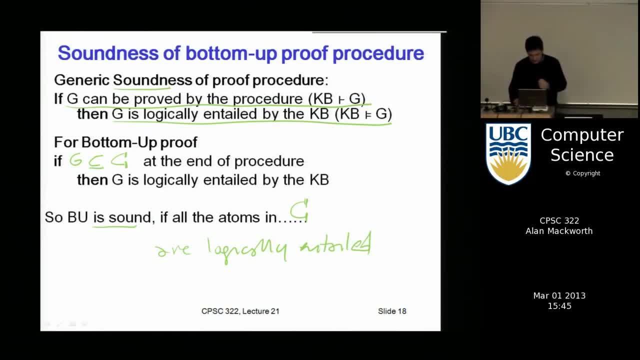 it should be kind of clear. ok, so what we want to prove is that all the elements of c are logically entailed. ok, yeah, is g the true set of atoms that can be derived, or no? no, g is something we are. we are asking: is this derivable? 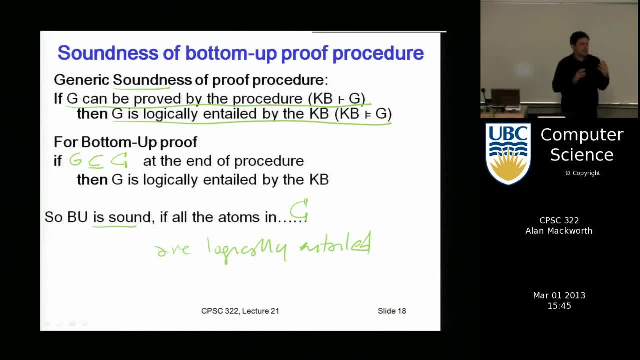 oh yes, and the proof, the proof procedure is saying: g is derivable, this is a. if it's a subset of c, ok, ok, so we are. we are proving this by contradiction. you already saw the proof of like a star optimality: by contradiction, and again it's a. 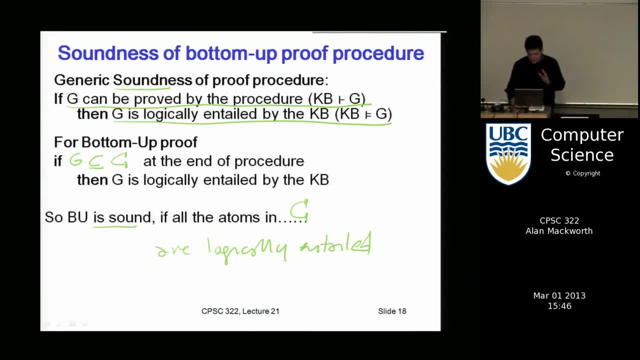 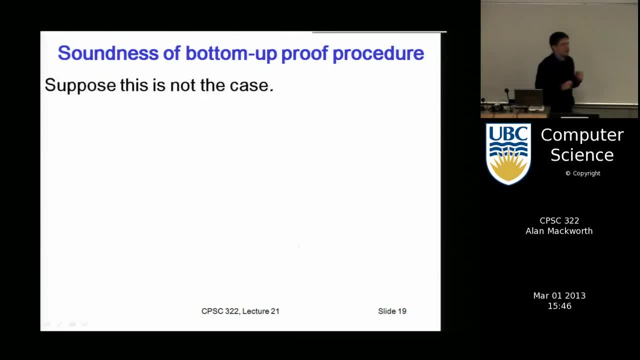 it's kind of a meta proof. we are proving something about the proof, but hopefully, by breaking it down it's going to be to digest. so let's assume that this is not the case. one is not the case that not all elements of c are logically entailed. 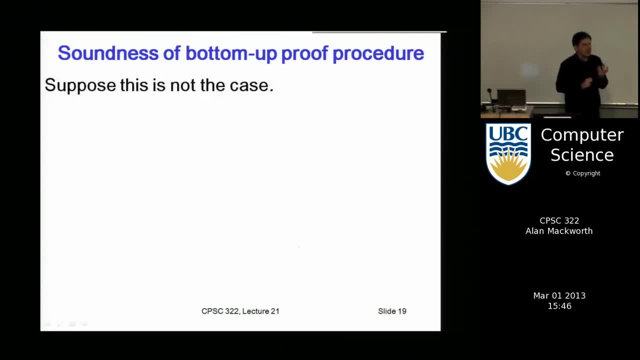 so the way for this not to be the case is that, at a certain point, this proof procedure is adding something to c that is not logically entailed. ok, so let's focus on this step, this, when it's doing, it's making a mistake. so h, let's consider h. 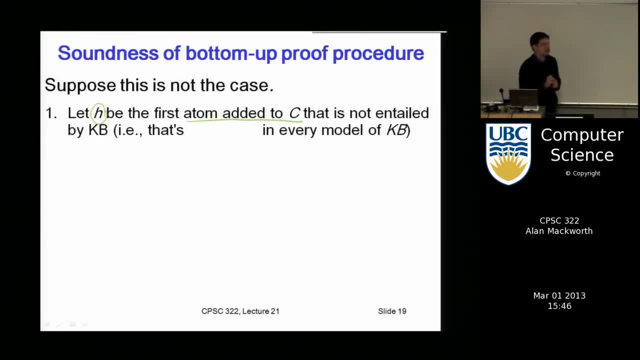 be the first atom added to c that is not logically entailed, because we are assuming now that they are not logically entailed. so at a certain point the procedure is adding something that is not logically entailed. so if it's not logically entailed, then h. 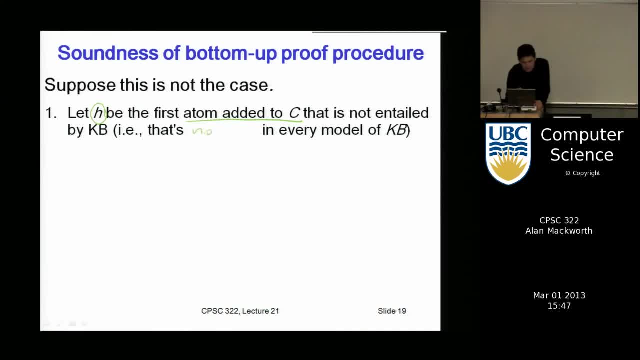 is not true in every model, ok, if it's true in all the models, it's logically entailed. so in this one model it might be false, ok, ok. so let's say: well, there is a model in which it's not, it's not true, and let's call this. 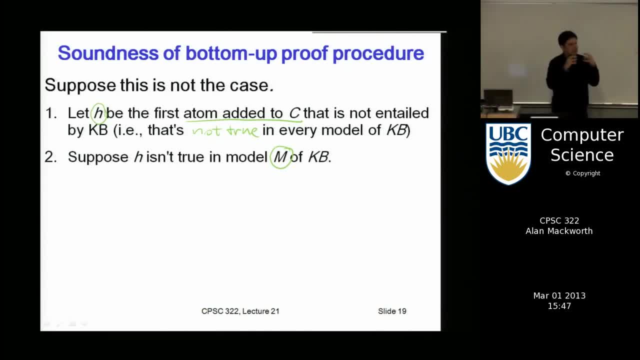 m. so at this point we are reasoning about the semantics, what it means to be logically entailed. ok, so now let's go back to the procedure. we are adding h. the bottom up procedure is adding h. when h is added, well, there must be a clause in the knowledge base. 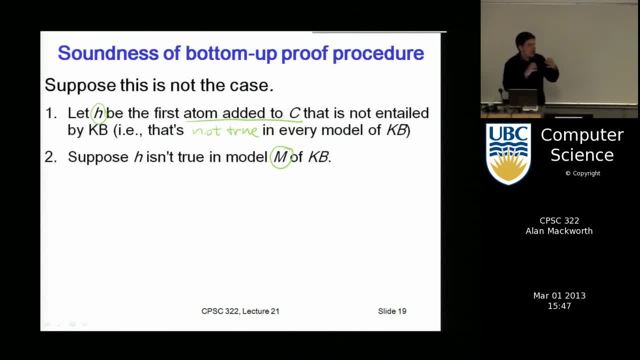 with h as an add. so that's how it works. a new add, a new atom, only if there is a clause in the knowledge base and the antecedents are already seen. ok, so h was added, was added to c. there must be a clause in the knowledge base. 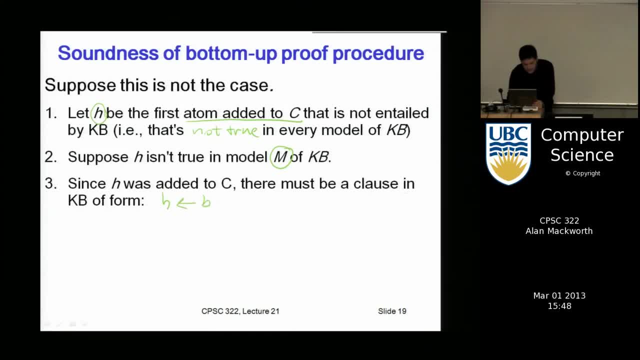 of the form h, multiplied by d, 1 m. ok, so now we have a clause in the knowledge base that has this body. and then there is h as the, as the consonant. ok, but now h d i is subtracted from h, so h d i. 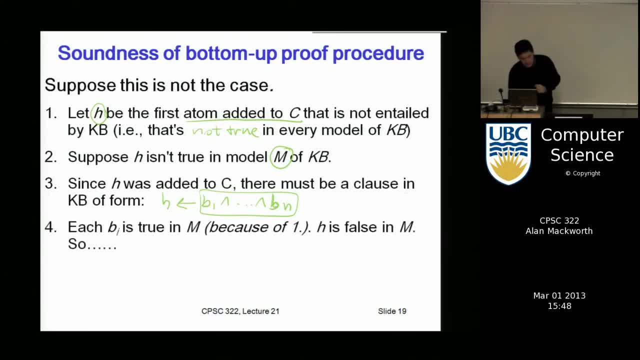 is subtracted from h, d i is true, must be true in m in the model. why? because, remember, we started saying this: h is the first atom that was added to c, that is not logically entailed. so all the antecedents of this rule, they already. 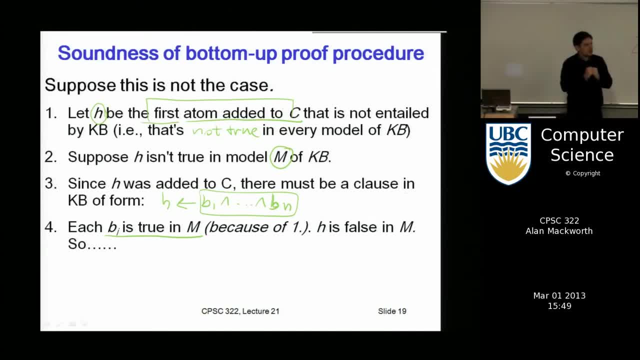 have. they have to be logically entailed by the knowledge base. ok, so h is the first one that we are, that we are adding. ok, so we have all these that are true in this model because they are logically entailed, so they are true in the model. 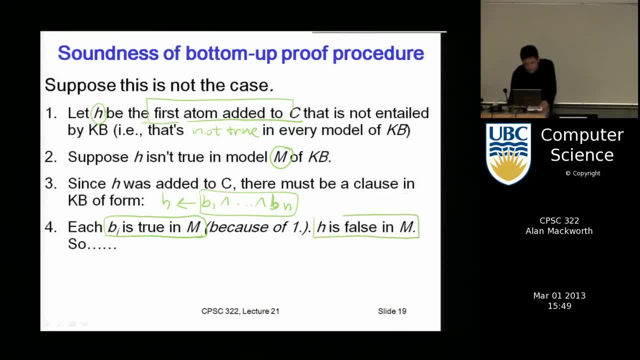 h is false in the model. so that's what we derived. we say it's not logically entailed. we pick exactly that model in which it was not. so what we have? we have a rule in the knowledge base for which the antecedents are true but the consequence. 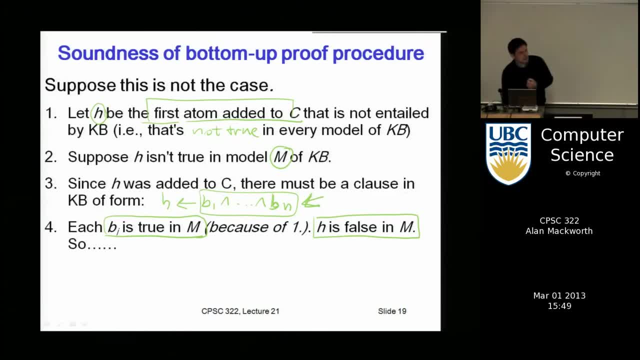 is false in that model, in that interpretation. that's called interpretation, because if you have a rule in the knowledge base of which, for an interpretation, the antecedents are true but the consequence is false, that cannot be a model. ok, because remember the clause, every model in the knowledge base. 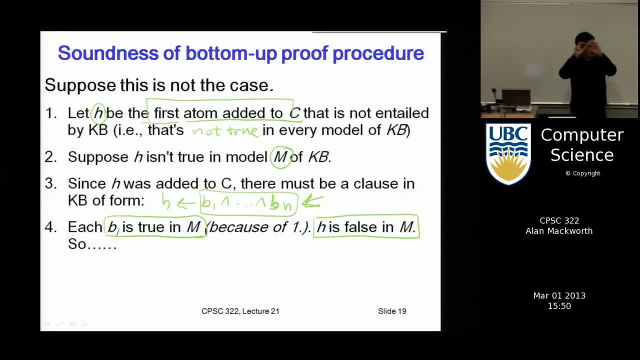 for a rule: the body cannot be true and the consequence be false. ok, so m is not a model. ok, so if n is not a model, then the cannot be true that we are adding something that is not logically entailed. ok, so we started by saying: if we add something, 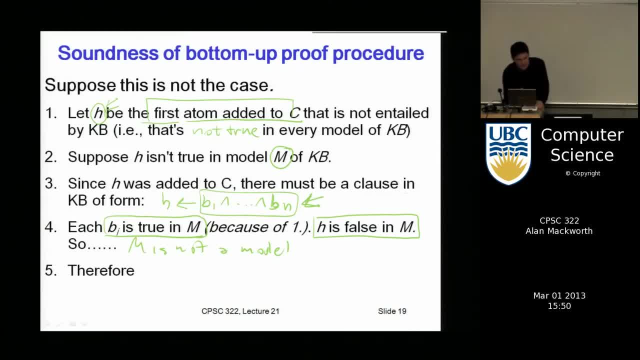 that is logically entailed. that is not logically entailed, then there is a model in which it is true, and then we prove that that's not a model. that cannot be a model. so it cannot be true that h is not logically entailed by the knowledge base. 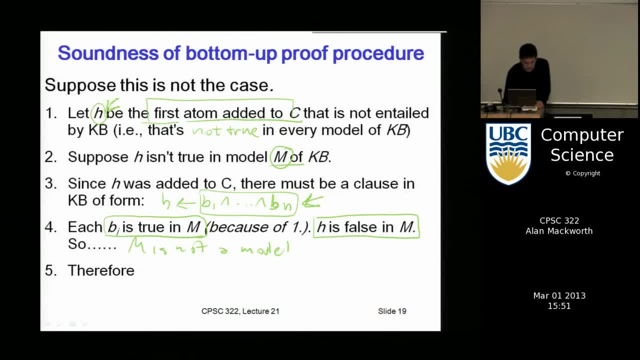 ok, so h must be. if we assume that at a certain point we are adding something to the, to c, that is not logically entailed, then we take the model in which that particular atom is false. but then we prove that that cannot be a model. so we have. 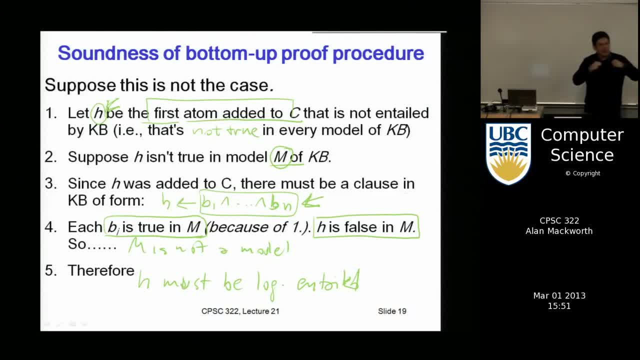 we have reached a contradiction, so we we just say that it's not a case, it's false. ok, so we have. we have reached a contradiction, so we we just say that it's not a case, it's false. ok, so you can go to the proof. it's complex. 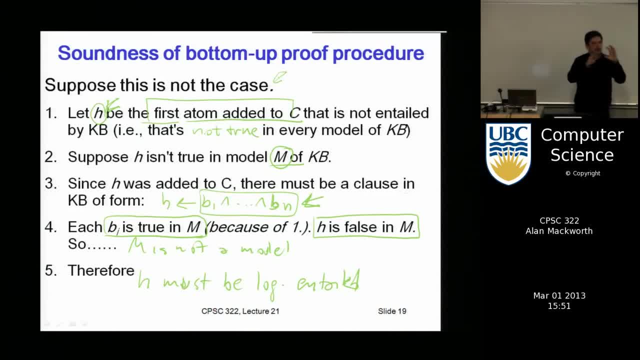 because it's mixing syntax and semantics and all the concepts that we have seen. but by proving this, we can be sure that whatever is derived by bottom up the procedure that we have seen is logically entailed, which is something that you need to do for any good procedure. 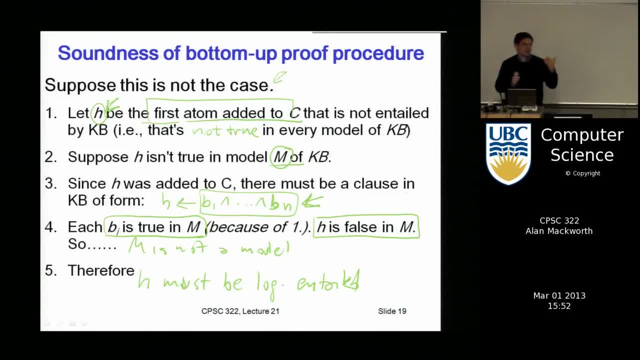 and next week you are going to see the counter function to show that everything that is logically entailed can be derived by the, by the proof procedure. ok, any questions on these? on these steps, it might take a while, but make sure that to get the full, but make sure.